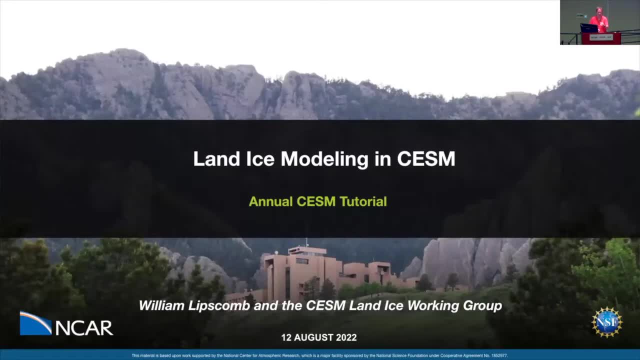 Good morning everybody. This is the first talk I've given in person in a really long time. It's good to be back in a real live in-person meeting again. So, as Peter said, I'm one of the main developers of the land ice component of CESM. 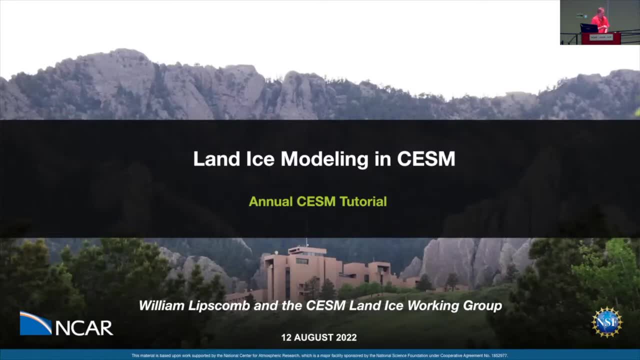 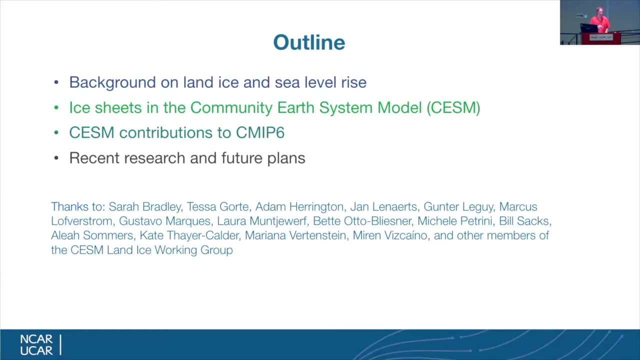 Okay, got it. So CESM is ongoing and what we'd like to do in the future as we work on work towards CESM 3.- And this work is the that I'll be showing is a combination of the work of a lot of people in the land ice working group, some of whom are listed here. 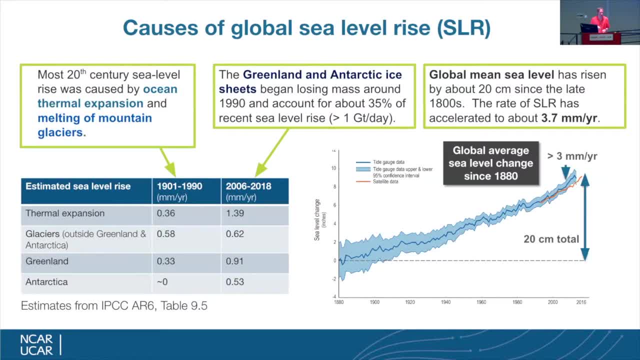 So everybody's aware that sea level is rising. Sea level has been rising since the steadily since the early 20th century, with significant acceleration toward the land ice. So since sea level has been measured by satellite since the early 1990s, the rate of sea level rise has been upwards of three millimeters per year and is now about 3.7 millimeters per year. 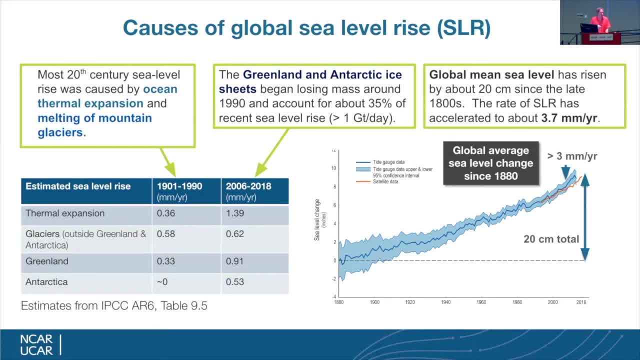 With three primary causes. One is the ocean: thermal expansion. ocean ocean water gets warmer, I mean gets less dense as it gets warmer. Second, there's been ice loss from nearly all the mountain glaciers of the world. And finally, in recent years, since about the 1990s, there's been a significant sea level contribution from the two ice sheets Greenland and Antarctica. 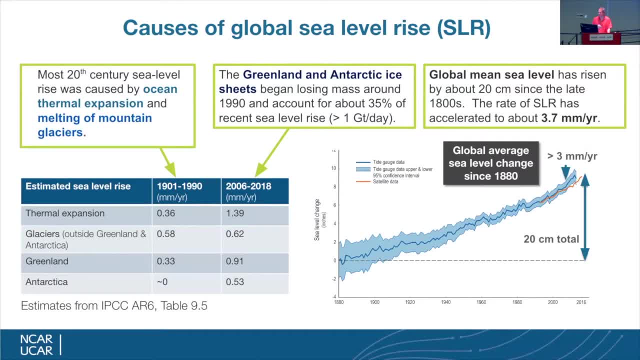 And currently, if you look at the contributions from each ocean, thermal expansion, mountain glaciers and ice sheets, each accounts for about a third, or roughly a millimeter per year, of the observed sea level rise. And if you just to put this in perspective, one millimeter of sea level rise may not sound like a lot, but it represents about. 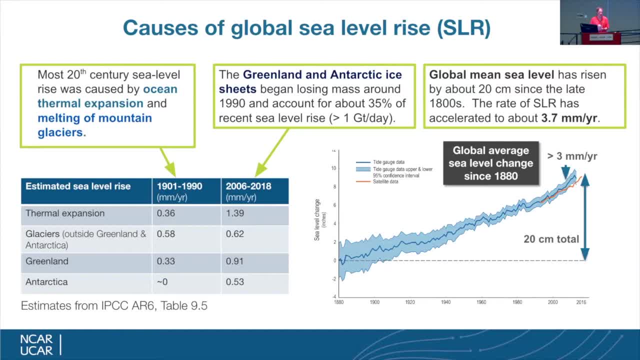 360 billion tons of ice and 1 billion tons of ice is, if you can imagine, is an ice cube. that's one kilometer in each side. So if you think of an ice cube, it's one kilometer in each side. That's roughly how much water ice sheets are adding to the ocean on a typical day. 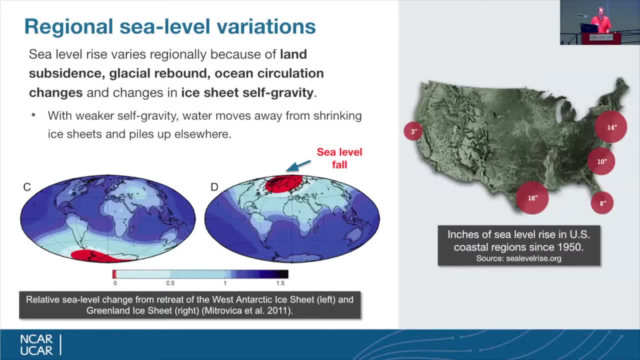 Sea level. I've given the numbers for global mean sea level rise. but sea level rise Varies a lot over time and over space For different reasons. locally you may have land subsidence that contribute to sea level rise. Some places are still rebounding from the last glacial period, which tends to contribute to sea level fall. 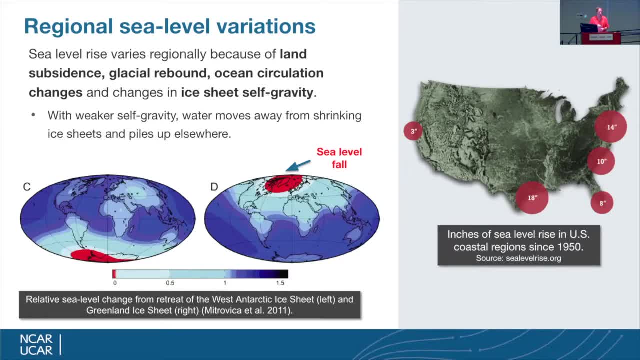 Also, as an ice sheet loses mass, it's less massive and therefore has less gravity, And so one of the sort of counterintuitive effects of sea level change is that, if you look at the pictures on the left, the red regions are where sea level is actually falling, because the ice sheets in those regions are no longer tugging on the surrounding ocean as much as they were, and and that's actually a negative effect on sea level rise that models are, most models don't yet take into account. 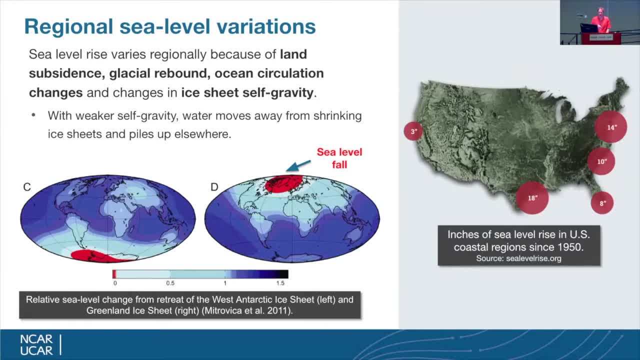 So if you look at sea level rise in the US, because of changes in ocean dynamics and other things, as well as the isostatic rebound, Sea level rise tends to be higher on the east coast than the gulf coast coast and the gulf coast than it is on the pacific coast. 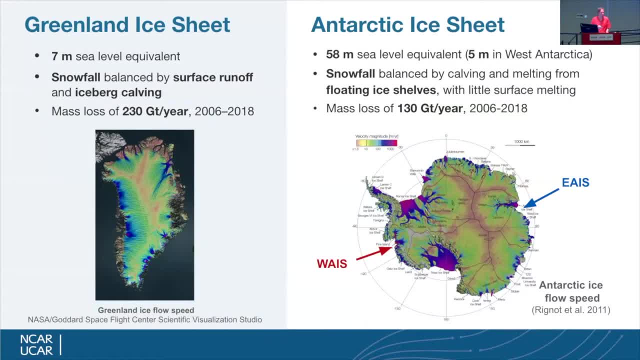 so the earth today, of course, has two major ice sheets: in greenland, antarctica, the greenland ice sheet. if you were to take all the ice in greenland and put it in the ocean, it would raise global sea level by about seven meters. and in greenland, before climate change, the well, most of the 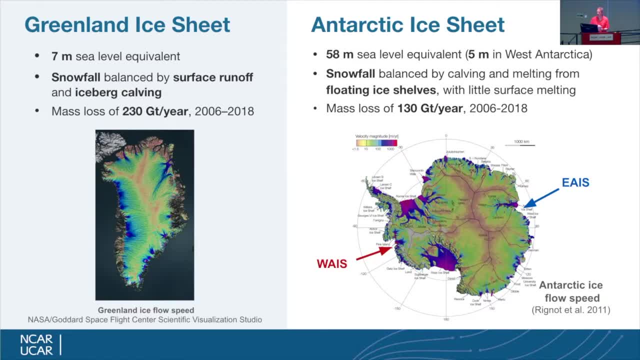 mass that arrives in greenland, of course, is by snowfall, and mass is lost by two major mechanisms, which were roughly equal before the climate started to warm. one was surface melting in the summer in the warmer parts of greenland, especially on the on the western slope in lower elevation. 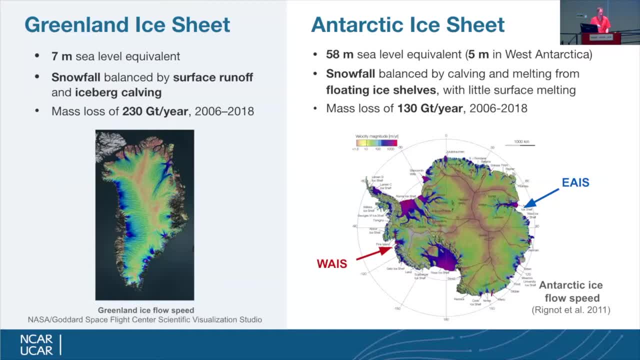 regions and then the other is calving of icebergs from outlet glaciers that flow through fjords into the sea and those processes were in balance until about the 1990s. now are out of balance primarily because of the climate change and the climate change in greenland and the climate change in 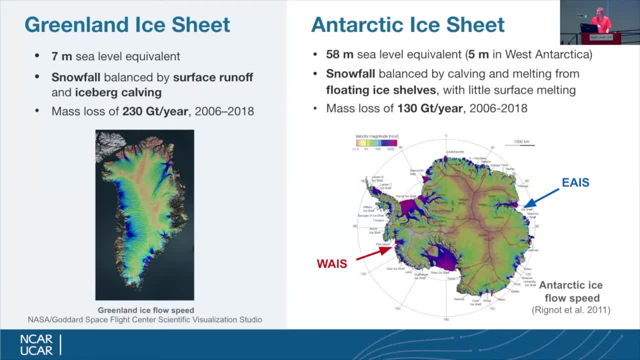 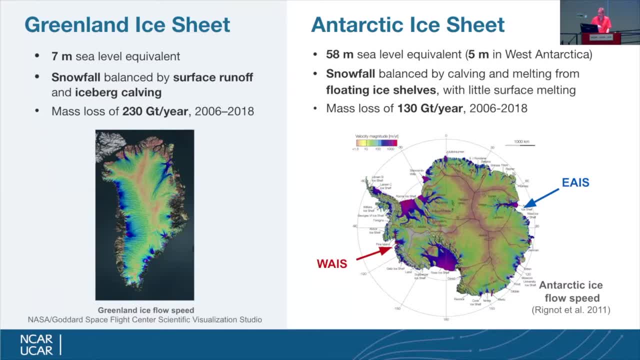 this the year we're in right now having greater, greater mass loss. most of the world's fresh water in the form of ice is locked up in the antarctic ice sheet, which contains about 58 meters of sea level equivalent. most of the antarctic continent, including the east antarctic ice sheet on the 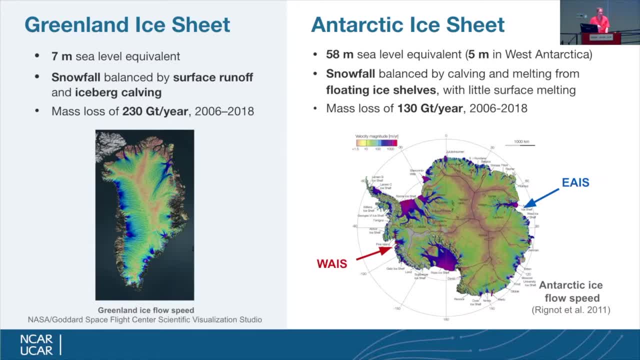 the right hand part of the picture is very high and very cold and not considered vulnerable to global warming of a few degrees or you know anything in the in the foreseeable future. however, the west antarctic ice sheet or waste in the left hand part of the picture. 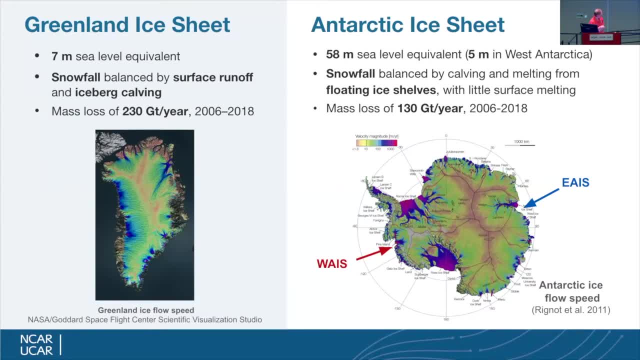 the majority of waste is grounded below sea level, meaning that the the marine grounded ice that forms waste and parts of the east antarctic ice sheet as well, is vulnerable to ocean warming, because if you have warm ocean water, even one or two degrees above freezing, that gets underneath the ice shelves that bring the ice sheet, you have the 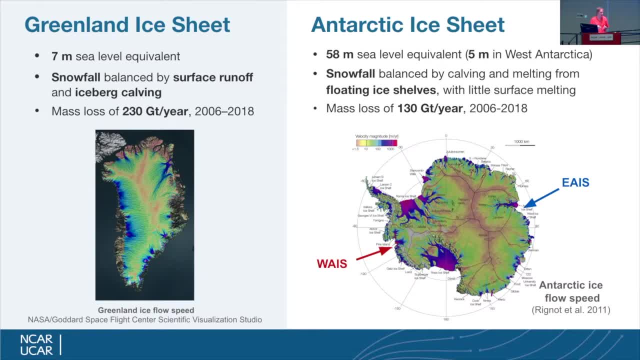 possibility of removing the ice shelves, thus reducing the buttressing that they provide to the grounded ice and having more grounded ice flow into the ocean, and it's the grounded ice that contributes to sea level rise. this has been happening in the last couple of decades, in recent years, primarily in the amazon sea embayment, which is more or less where that. 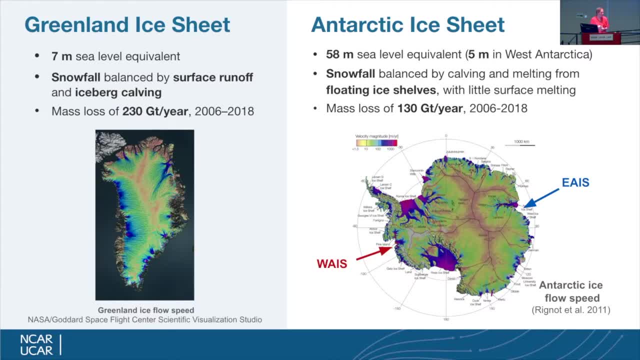 red arrow is pointing. you may have read in the papers about the pine island, thwaites glaciers, which are losing mass, and antarctica is losing mass currently by about 130 gigatons per year. so if you add the two ice sheets together you get about 360 or or about one millimeter of sea level. 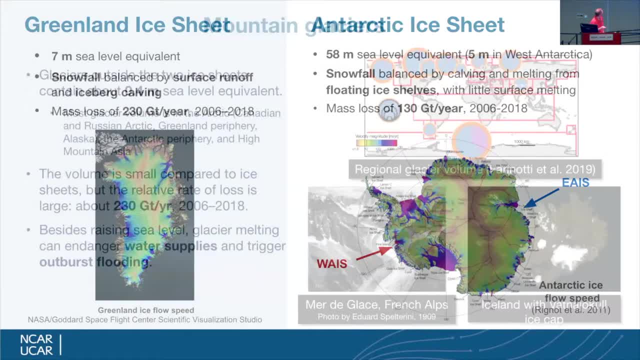 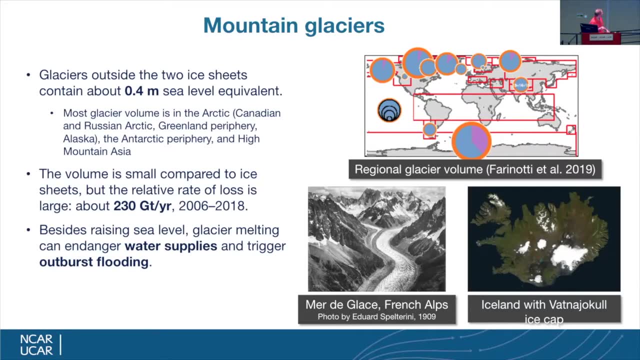 rise each year. then the other main contribution of land ice to sea level rise comes from the rest of world's glaciers. the map in the upper right shows circles corresponding to each of the major glacier regions as they're classified in something called the randolph glacier inventory, which is an 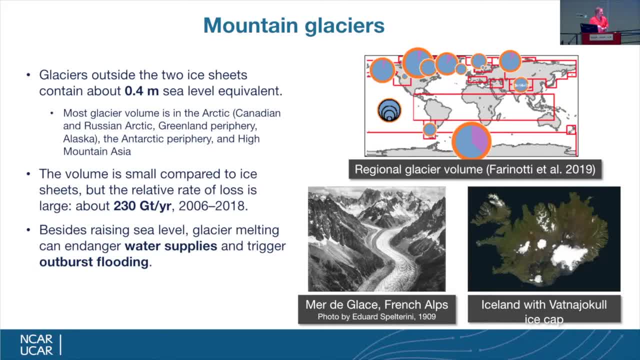 inventory that came out 10 or 15 years ago of all of the earth's roughly 200,000 glaciers and what their outlines were: their extent around the year 2000 or 2005, which is taken as a baseline of what the world's glaciers have been in retreat. most of the mass is in the high arctic. 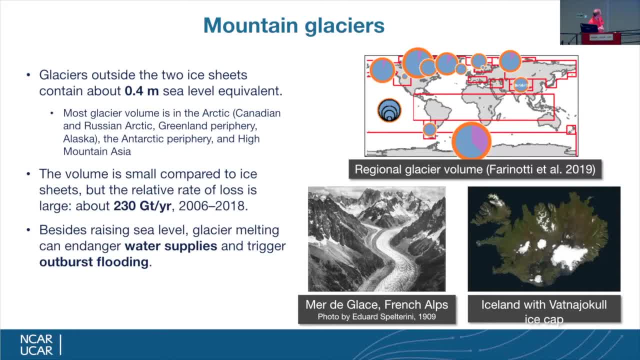 canada, greenland, russian islands and in the periphery of the antarctic ice sheet and then outside the poles of the place with the places with the most glacier ice would be high mountain asia in the himalayas and nearby ranges. if you add up all that mass. 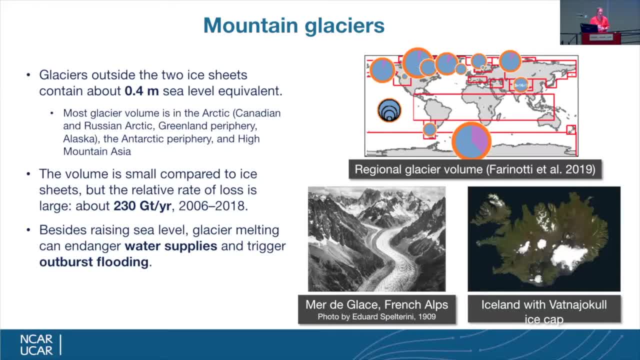 it only amounts to about 40 centimeters of sea level rise, so much less than in the major ice sheets, but since that ice is melting relatively quickly, the glacier contribution to sea level rises today is comparable to that of ice sheets, and in most of the world's glaciers are currently 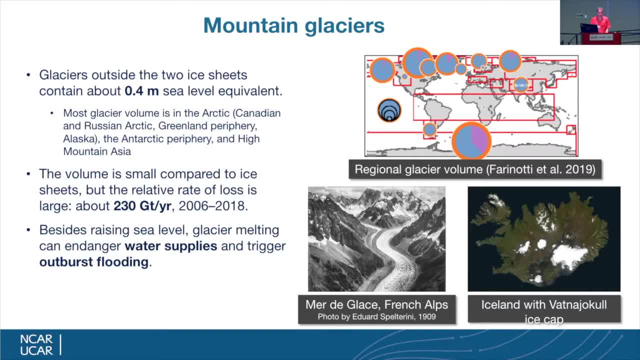 threatened and many of them could go away under in this century, under warming of well either under, even if there were no additional warming. many of those glaciers are threatened and more will go away if warming continues up till up to one and a half or two hundred percent of the world's. 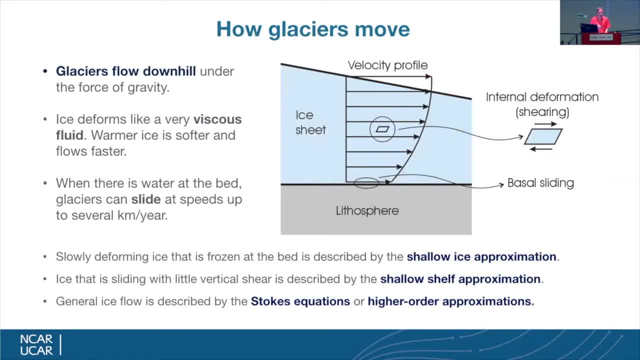 two degrees. so a little bit about glacier dynamics. glaciers, of course, don't move very quickly compared to other parts of the climate system, but they have two main mechanisms of moving under gravity. one is if a glacier is frozen to the bed. a glacier can be described as a fluid and 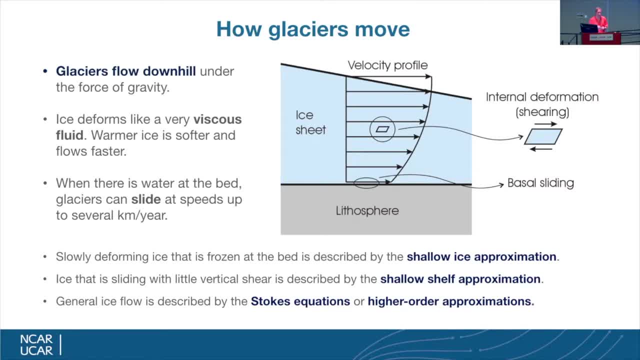 it deforms slowly under its own weight and can flow at rates of a few meters to a few tens of meters per year, or by by internal deformation, with the greatest speeds being at the top of the glacier and the lowest speeds being at the bed of the glacier, but then in places where the glacier, where glaciers have 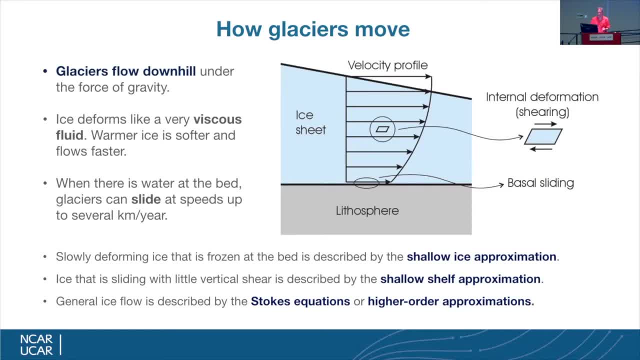 been relatively quickly, and relatively quickly for a glacier would be anywhere from a few hundred meters to a few kilometers per year. that's the case when the bed is lubricated, when there's water at the bed or when the soil beneath the glacier is water saturated and weak. and if you 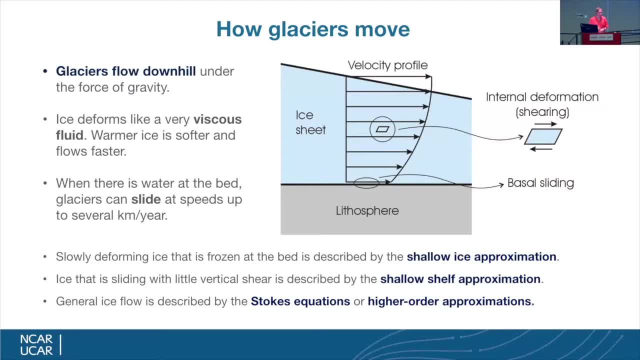 have a glacier sliding, then you can have speeds of above a kilometer per year and the big glaciers that are losing mass. that's that's definitely the case. if you have ice that's slow moving at the bed and deforming mainly in in the interior under its own weight, then it's described very accurately by a set of 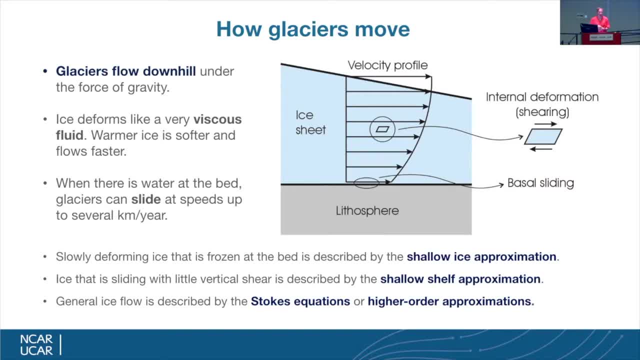 equations called a shallow ice approximation. and if you have the opposite situation, where you have no friction at the bed to hold the ice and the entire ice sheet is going to be in the middle of the bed moving, or ice shelf is moving like a plug with no vertical shear, then that's very well described. 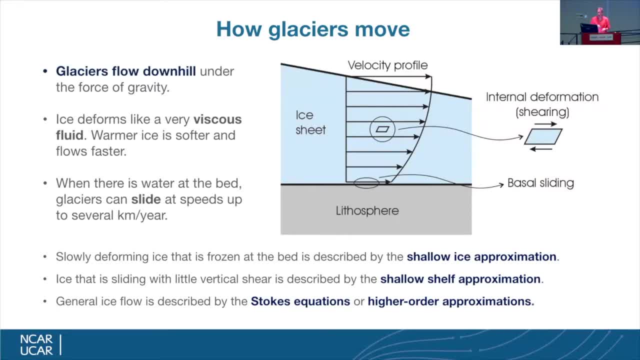 by something called the shallow shelf approximation, and both those approximations are fairly straightforward to solve mathematically on a computer. but the more general set of equations is called the stokes approximation, where you have all kinds of internal stress that's causing the movement, and those equations are much more difficult and expensive to solve and as a 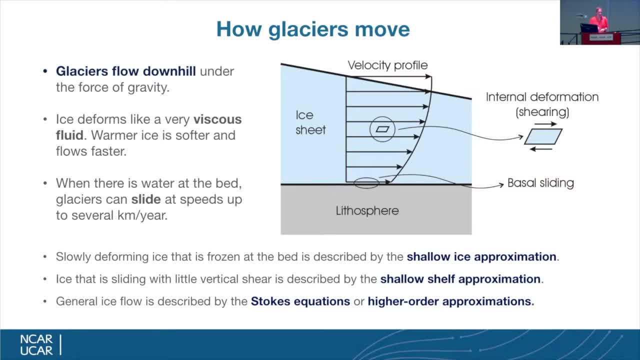 compromise. we typically use what are called higher order equations, and those equations are approximations where we start with the more complete stokes equations and remove some terms that make the equations harder to solve and are left with something that's more computationally tractable but still include both this shallow ice approximation, the shallow shelf approximations. 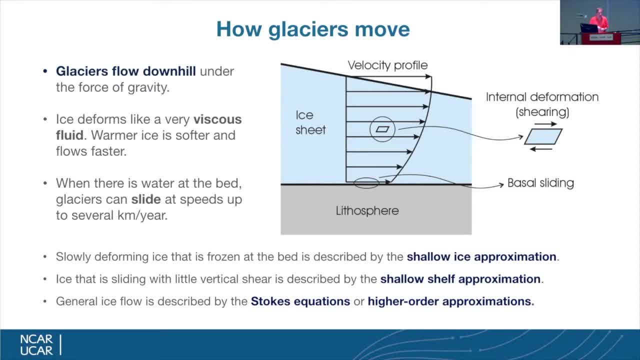 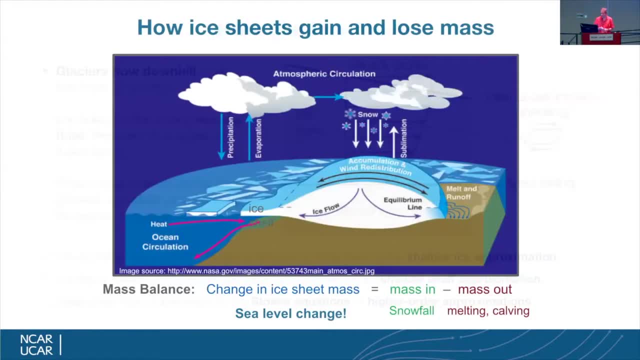 endpoints in the appropriate parts of the ice sheet, so on the community ice sheet model, sysm. that's the approach we usually take for for production runs, and then ice sheets, as i said, are losing mass currently. it's important to keep in mind that that a melt event on an ice sheet like greenland 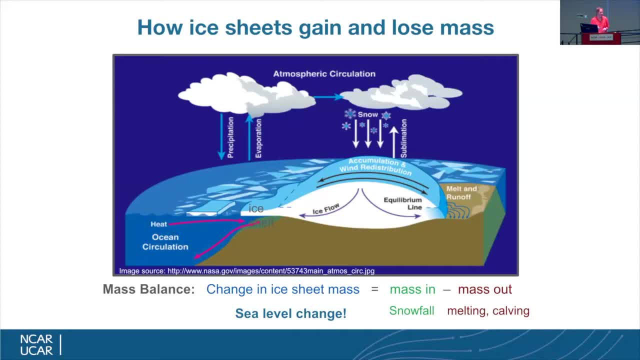 is not in itself an indication that the climate's warming, because there were melt events in greenland before climate change, but what we're seeing now is more frequent and much more intense melt events. such the system's out of balance, such that the snowfall that comes in annually is less than the 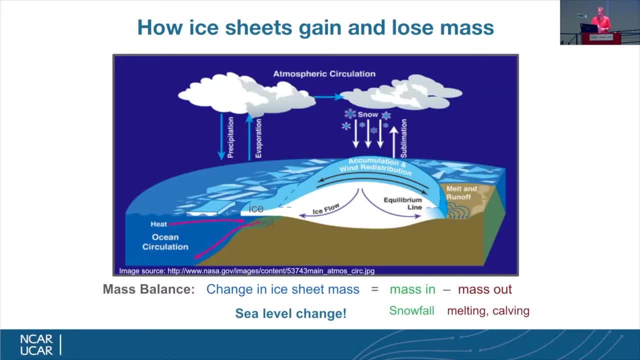 mass that's lost in greenland in the summer to to surface melting. so you typically would think that's the approach we're taking. but it's not the approach we're taking. we would have a balance between snowfall coming in and ice flowing into the ocean, and either 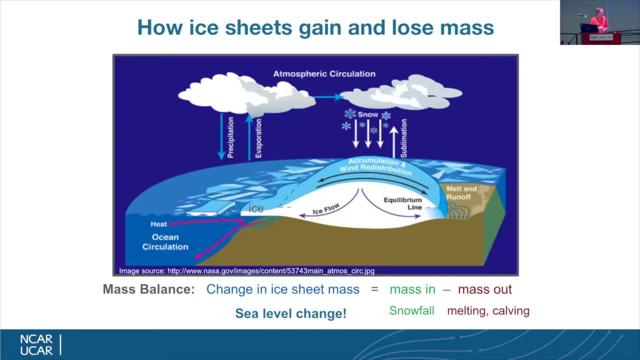 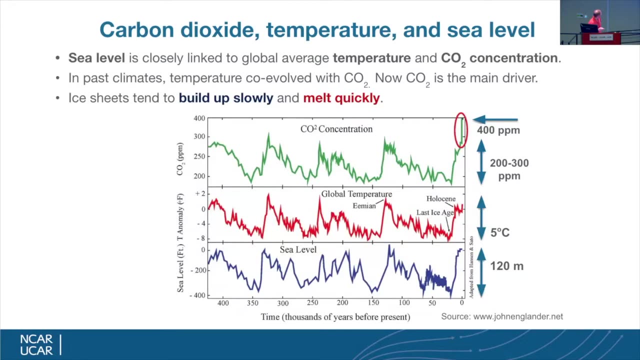 melting and having melt water run off near the coast, or the ice actually flows into the ocean and eventually calves off from an ice shelf. this is a plot you may have seen showing over the last 400 000 years, based on ice core evidence, how carbon dioxide and global mean temperature 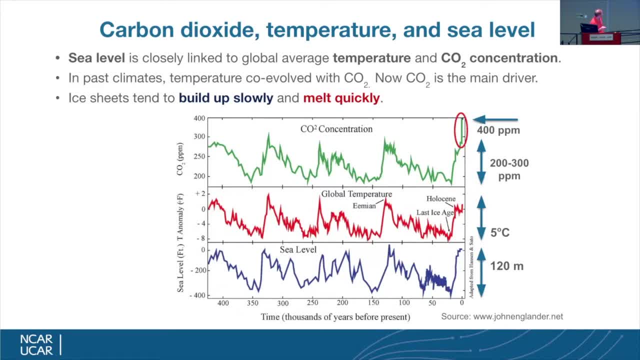 and sea level have changed simultaneously and you can see that they're very well correlated with each other, with sea level ranging by about 120 meters between the cold glacier periods and the warm interglacial periods. the most recent glacial period ended about 20 000 years ago. 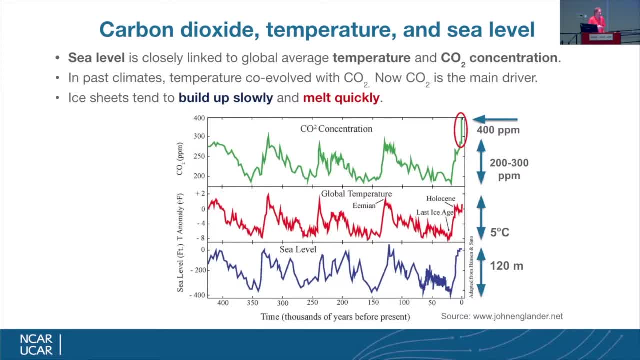 after the following the last glacial maximum and that was followed over the next 10 000 years or so by about 100 meters of sea level rise as the big northern hemisphere ice sheet collapsed and there may have- uh there may have been some additional retreat in antarctica, followed by some 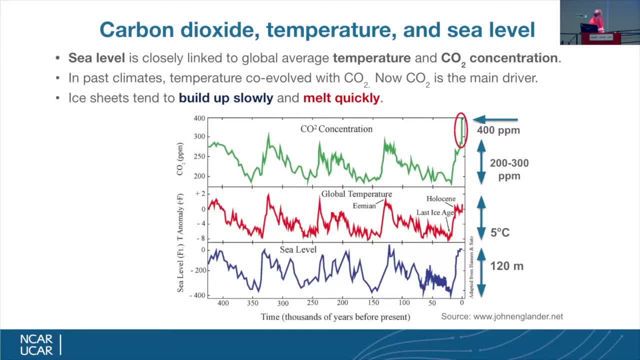 rebound, but it's um, but that's something people are still still debating about, um. at any rate, co2 and temperature were co-evolving, uh for most of history, before fossil fuels started being added to the atmosphere. now, of course, carbon dioxide is driving things, and we can expect that the 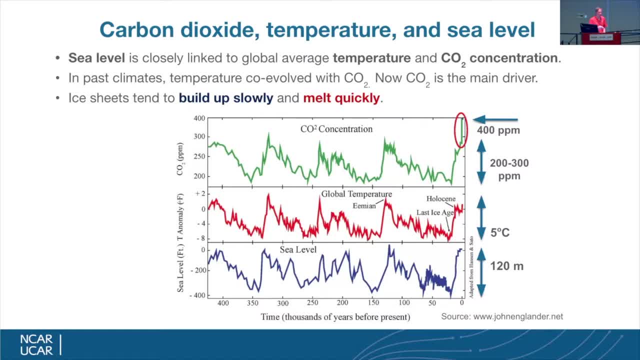 co2 of 400 parts per million, which is unprecedented, and we can expect that the co2 of 400 parts per million, which is unprecedented, and we can expect that the co2 of 400 parts per million, which is in it in more than a million years, is going to drive some additional sea level rise and, of course, 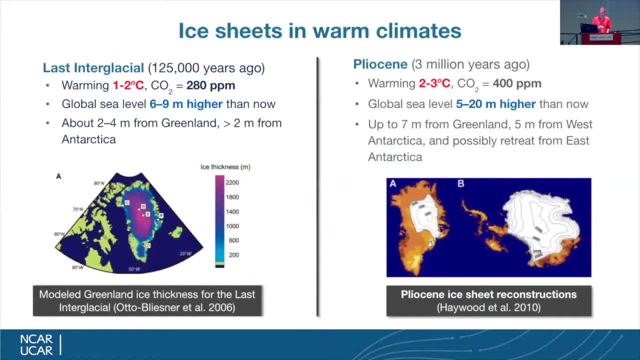 the question is how much? uh? so to partly answer that question, we look to past warm periods. uh, the most recent interglacial, called the last or emian interglacial, uh, peaked around 125 000 years ago. the earth was, on average, was, uh, maybe one, probably no more than two degrees celsius. 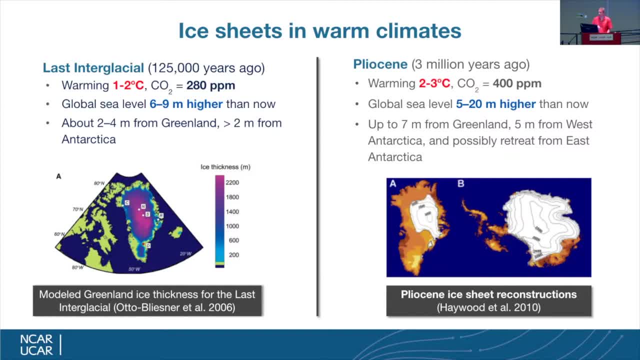 warmer than pre-industrial temperatures and carbon dioxide was around 280 parts per million, and evidence suggests that global sea level was somewhere between six and nine meters higher than it is today. so where did that six to nine meters come from? uh, we know that part of it came from greenland. uh, but we also know from paleo evidence that the entire greenland ice sheet 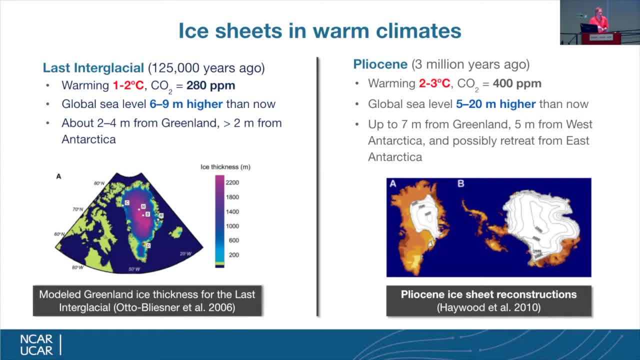 didn't grow away, didn't go away during the last interglacial um, maybe two or at most about four meters of sea level equivalent. so that suggests that to fill out the budget you need a sea level contribution from antarctica. and that's what we're trying to do. we're trying to make sure that we're. 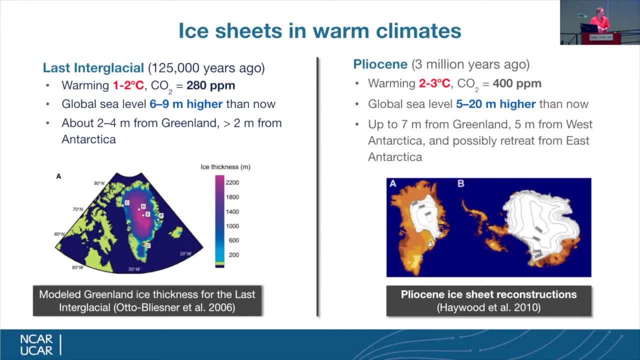 working our way through it, and i think that's one of the things that we're doing now for the final survey, the last few years, with what we're looking at is the state of climate change, and then the state of climate change is that we are talking about that international climate change. 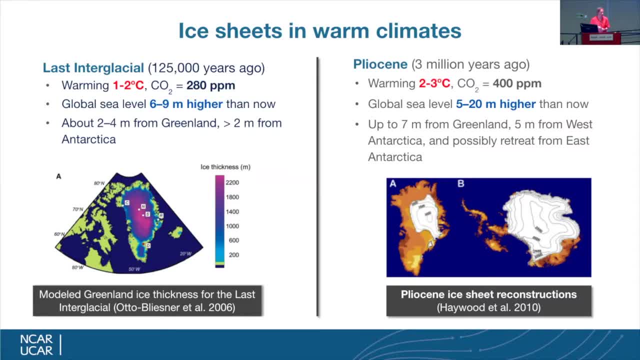 region and we're actually looking at the state of climate change as well- and that most likely came from the more vulnerable west antarctic ice sheet. so we know that both greenland and wastes are vulnerable to sustained warming of of something in the neighborhood of one to two degrees, which is 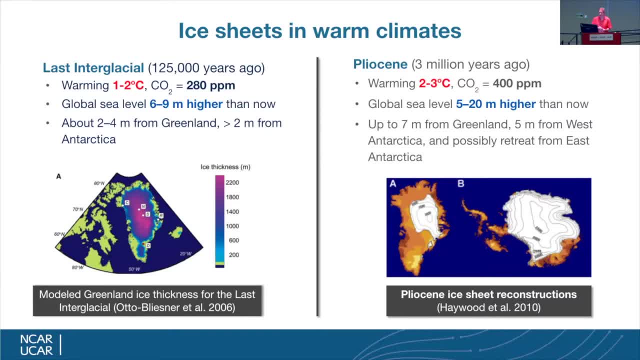 where we are now and heading into in the next few decades. the last period with co2 comparable to today's levels of around 400 ppm was the plyo scene about two to three million years ago, and there the paleo records are much less than the carbonley bins of the western pacific, and that's. 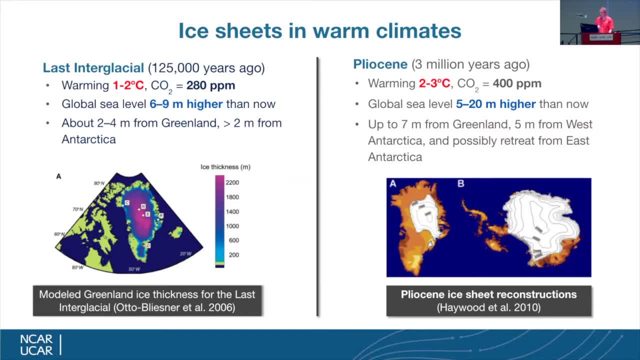 a think. that's a one-to-one comparison and you can't have a anymore transport of carbon في less certain in terms of what the total sea level rise was, with estimates varying anywhere from about 5 to 20 meters At the high end. you need a contribution, not just from Greenland and West. 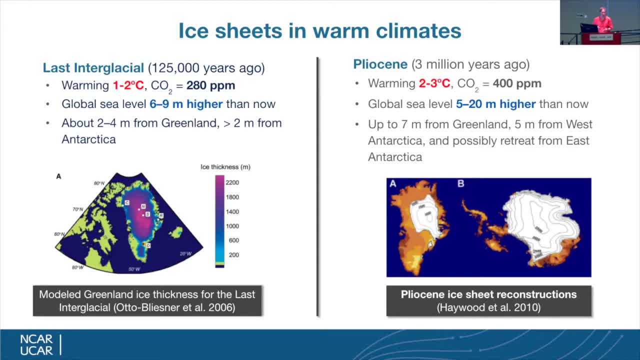 Antarctica, but also East Antarctica, And if East Antarctica too is vulnerable to CO2 of 400 ppm, that's obviously very worrying. So another area of active research is just how much sea level rise was there at the Pliocene, and is that something we could expect under temperatures? 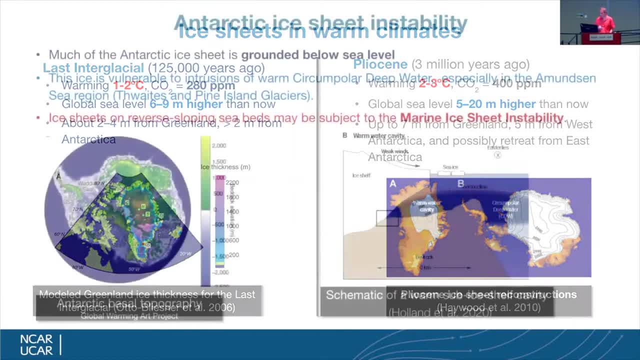 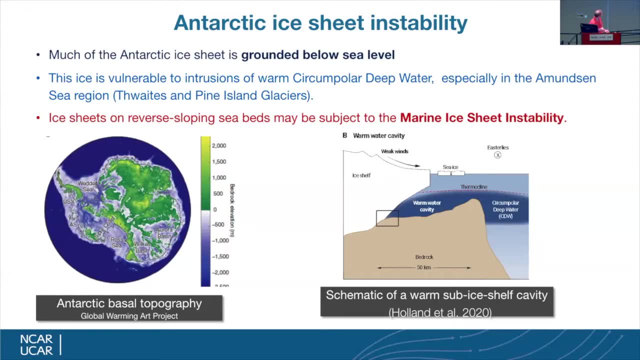 comparable to what we'll see later in the century. As I said, a lot of the Antarctic ice sheet, especially in the West, is grounded below sea level, So all the areas that aren't green in the left-hand plot are areas where the bed is below sea level and hence potentially 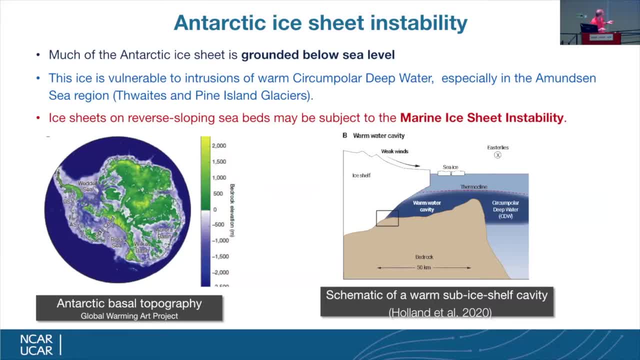 vulnerable to warming ocean water. The plot on the right shows a schematic where, in the Southern Ocean, the warmest water is typically not at the surface but at the subsurface, because it's more saline and dense than the cooler water at the surface. And so, if you have 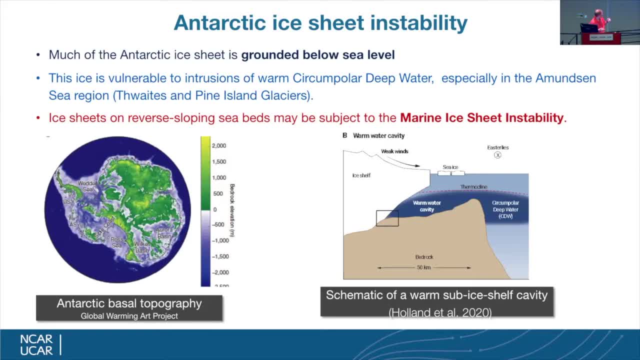 relatively warm circumpolar deep water that has access to an ice shelf cavity and is able to get into the cavity, it can warm the base of the ice shelf and start melting, And then after that, the geometry of the seafloor is very important because if the slope is like shown on the right, 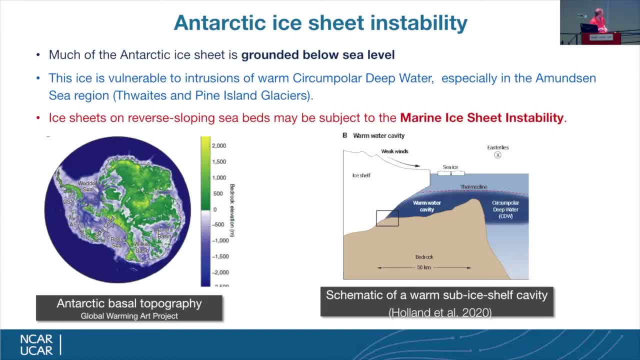 where you have the seabed going down as you go into the ice sheet interior, then the dynamics of ice sheet are such that the ice sheet gets thicker at its margin as it retreats, And if it's thicker it flows faster. If it flows faster, it thins. If it thins, then the margin is even. 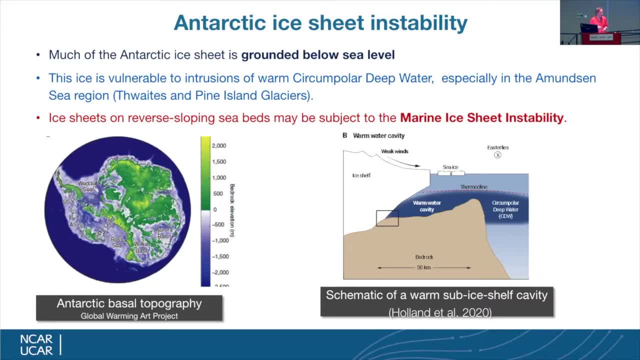 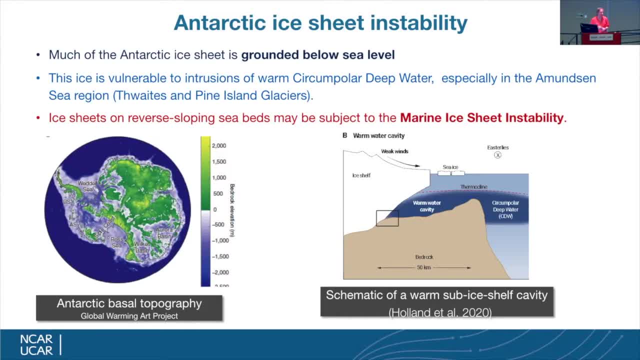 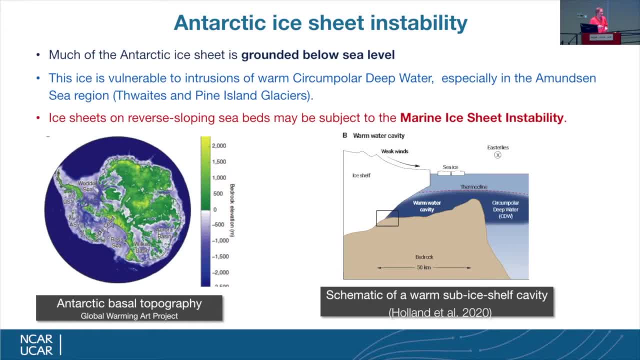 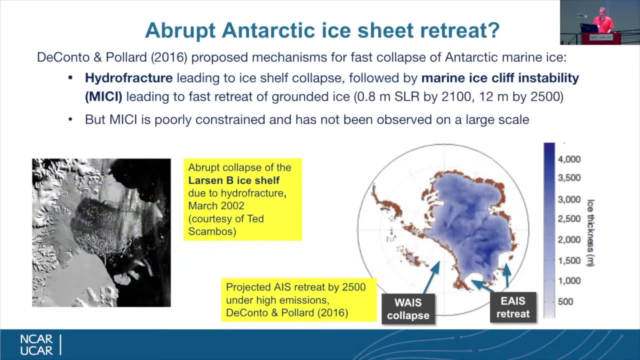 the schematic. So the worry is that once you start this process in motion, it may not be something that would stop, even if you were able to remove the forcing, And that's known as the marine ice sheet instability, or MISI. There's been a lot of publicity in recent years about other mechanisms for fast ice sheet retreat. 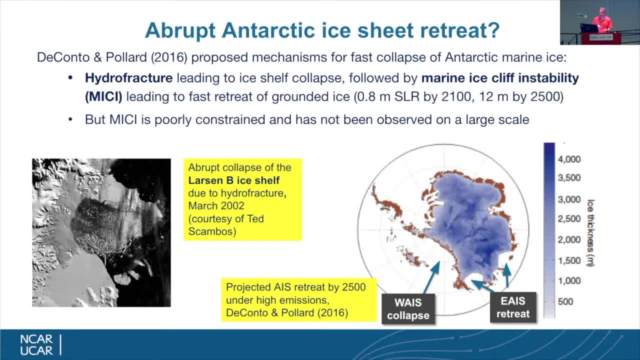 might work even more quickly than MISI. So MISI typically is relatively slow. It might remove a lot of ice in a timescale of several centuries. DeCanto and Pollard a few years ago in a well-known paper, suggested that another set of processes hydrofracture, meaning that you have 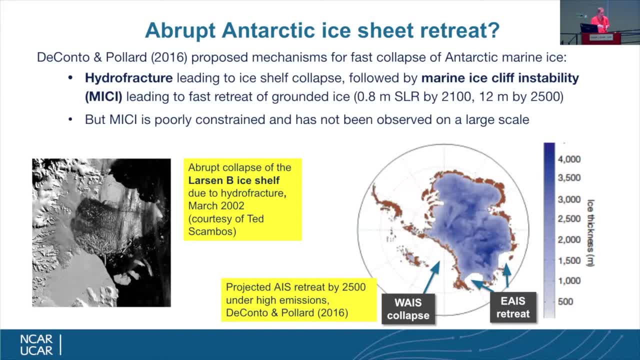 warm melt water in the surface of an ice shelf. that makes crevasses and can make the shelf unstable. Hydrofracture. combined with another mechanism they proposed called the marine ice cliff, instability could lead to fast sea level rise, such that you would have potentially 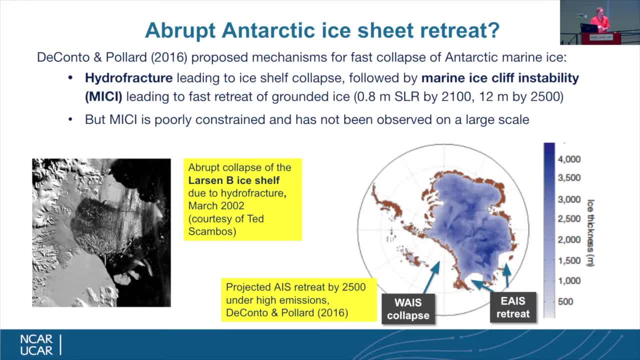 something to the order of a meter from Antarctica in the next century and maybe five meters from Antarctica over the next several centuries. However, MICI as a mechanism is not at all well understood and it's not something that's observed on any large scale, So a lot of people 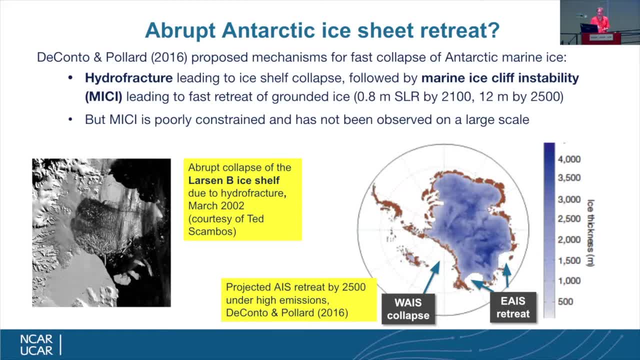 have said that it's not a mechanism that's observed on any large scale. So a lot of people have said: well, it's premature to suggest that a mechanism like this is going to be at work when we don't understand it very well theoretically and it's not something we currently observe. 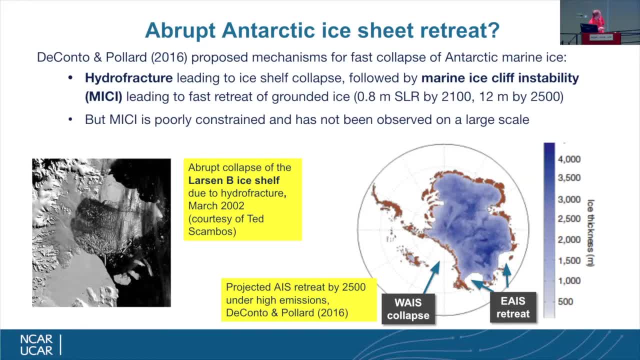 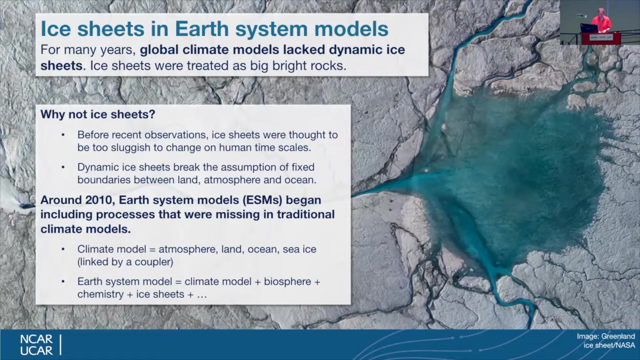 So I tend to be skeptical about it, but it is something that people are trying to build more complete models of and understand if it's a real threat to accelerate ice sheet retreat beyond what we think will happen with just the marine ice sheet instability. So now I wanted to say a bit about ice sheets and CSM Earth system models for many years. 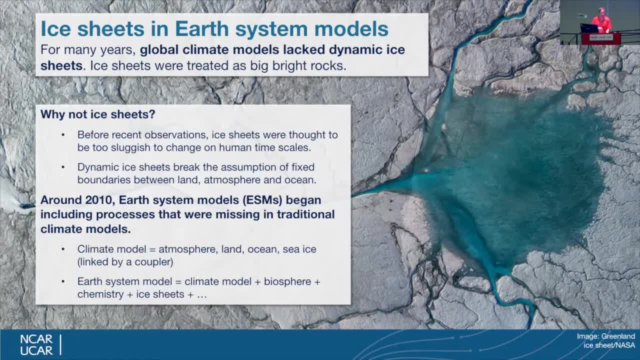 didn't have dynamic ice sheets, and ice sheets were just treated as basically big, bright, stable rocks and models, And this was partly because it was thought that ice sheets weren't going to respond very quickly to warming and partly because it's just incredibly complicated. 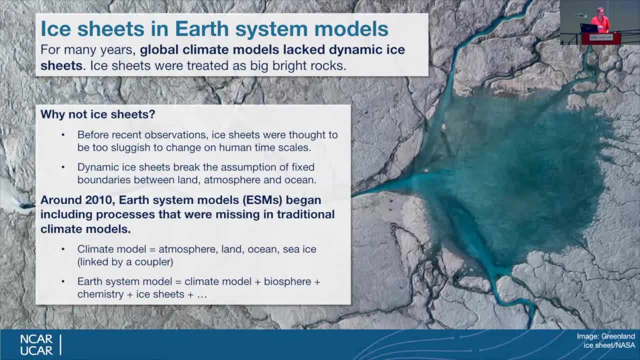 to put ice sheets in a climate model in such a way that the ice sheets are not going to respond to boundaries between land and ice and ocean are all changing around, But with observations earlier in the century that suggested that ice sheets are actually pretty dynamic and can change quickly. 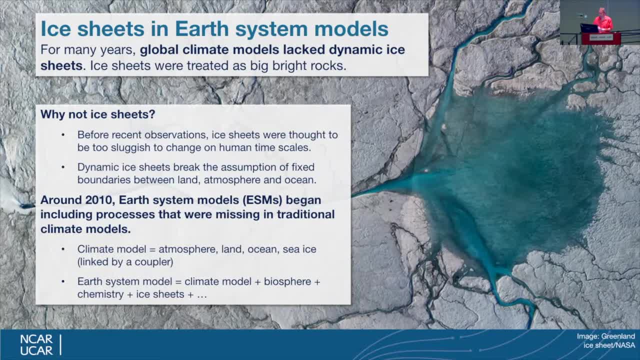 CSM and other modeling groups started modifying their models to include ice sheets, And this was part of a general broadening of the focus of climate models toward what we now call earth system models that include different aspects of the biosphere and chemistry, and so on. 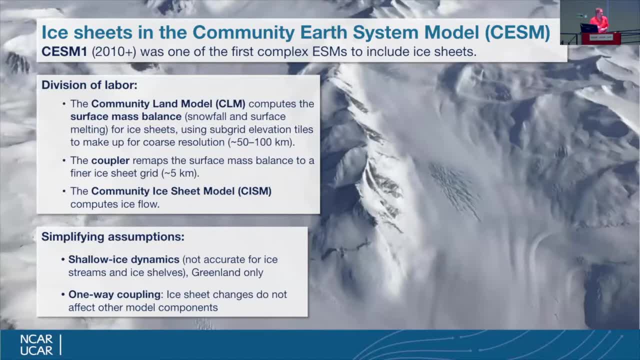 So in CSM we decided that the most efficient way to do this was to have the land model, CLM, or now CTSM, compute the surface mass balance of the ice sheet, meaning the snowfall and the later melting of the ice sheet, because CLM has more. 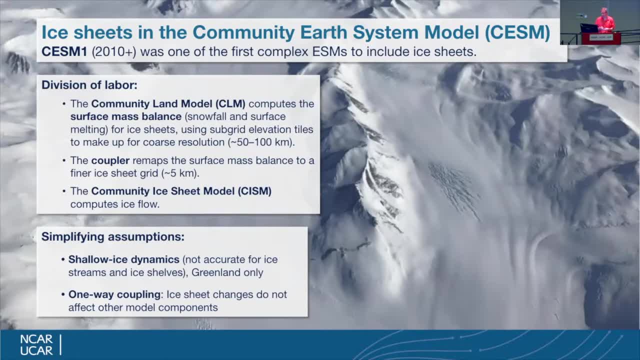 sophisticated snow physics and communicates regularly with the atmosphere. So the surface mass balance is computed by CLM and then remapped by the coupler to the community ice sheet model in an earlier version than we have now. In that earlier version we just assumed 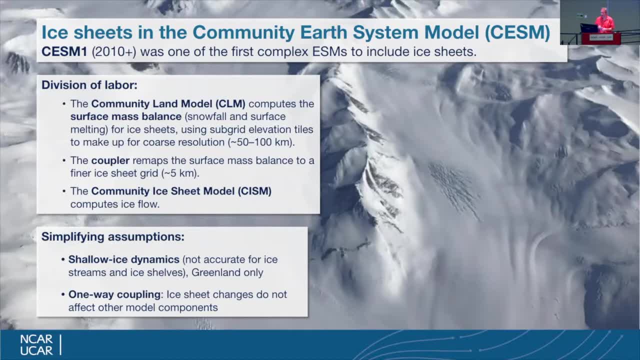 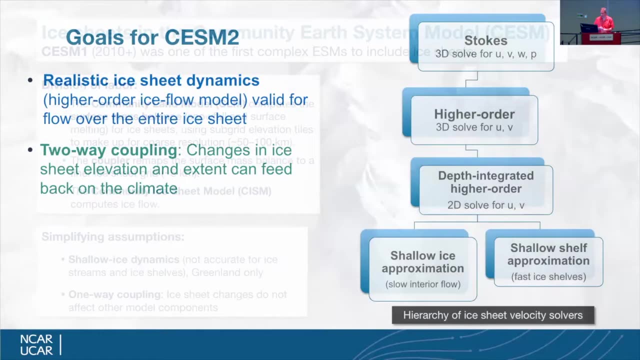 simplified shallow ice dynamics and only one way: coupling between the land and the ice sheet model. So the ice sheet model could respond to changes in surface mass balance, but changes in the ice sheet geometry didn't feed back on the rest of the climate. So for CSM2, which came out in 2018,. 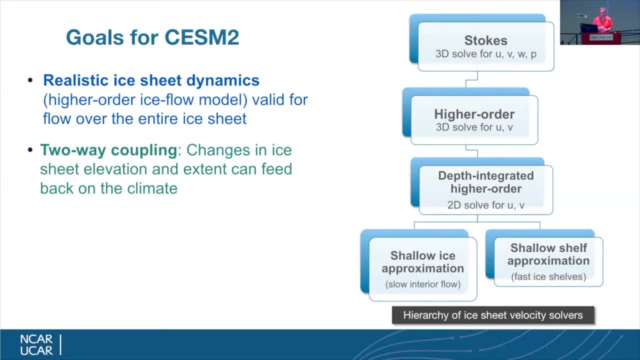 a couple of our goals were to make the ice sheet dynamics more realistic and also to allow changes in ice sheets to feed back on the rest of the climate. The plot on the right shows a hierarchy of ice sheet models, and what we usually use now is 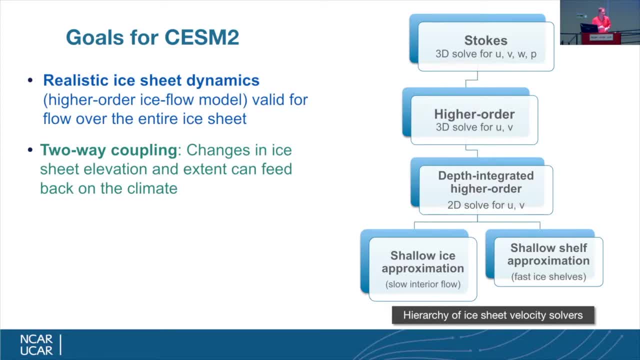 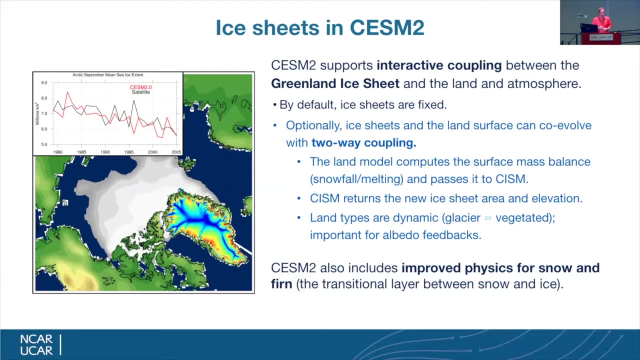 what's called the depth and graded higher order model, which is a nice compromise in terms of accuracy and computational costs between the expensive full stokes model and the cheaper shallow approximations. So in CSM2, if you just run CSM2 out of the box, the ice sheets are fixed. 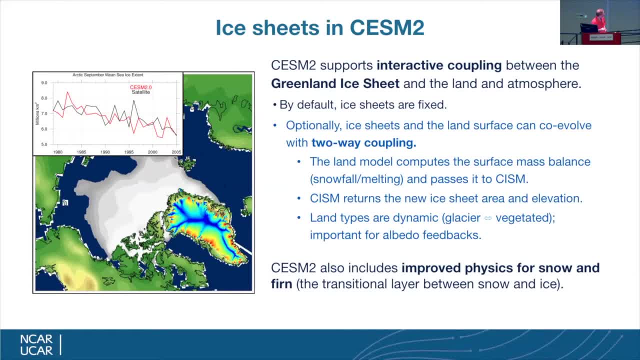 but if you set the ice sheets to evolve, you can get the Greenland ice sheet to evolve and as it evolves it will pass its new geometry back to the land model and the land model will then adjust. You may have heard that the land model has different land units: vegetated urban. 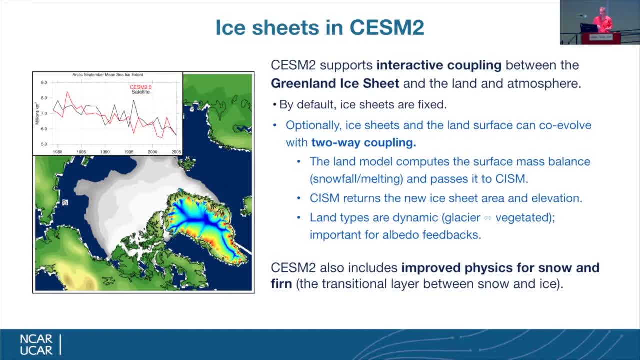 glacier and so on. And if you have an ice sheet, let's say that's retreating. then you have glaciated land units becoming vegetated and that's all handled under the hood in the model in a way that can serve the climate. So that's a good example of how the land model can be adjusted. 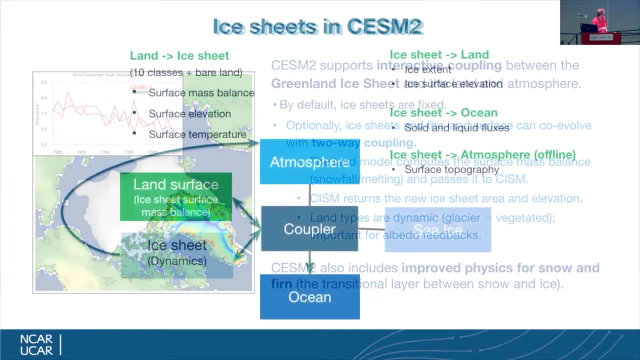 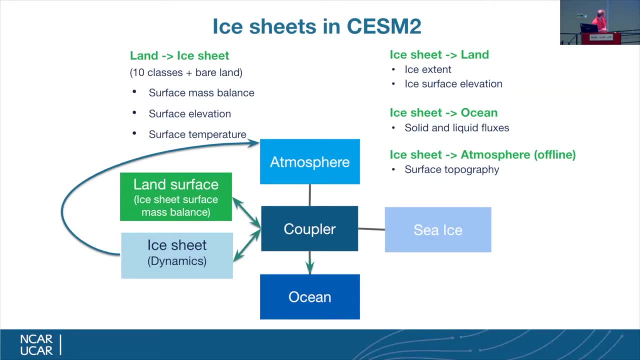 So this is a plumbing diagram just showing the parts of the model the ice sheets communicate with via the coupler. So the land model sends surface mass balance in different elevation classes to the ice sheet dynamic model and the ice sheet dynamic model will send. 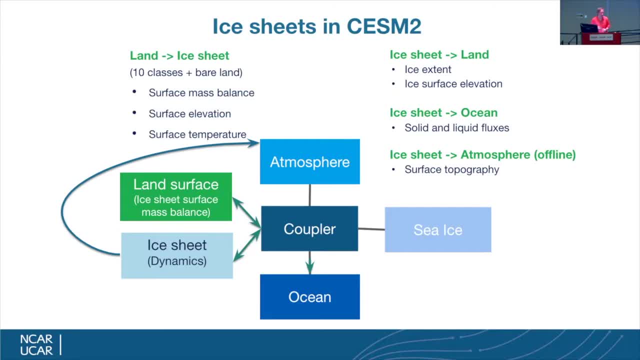 fluxes of either icebergs or liquid basal melting to the ocean. And then we don't have a way of changing the atmospheric lower surface topography on the fly during a run as, let's say, Greenland retreats, but we can do that offline, So you can stop the. 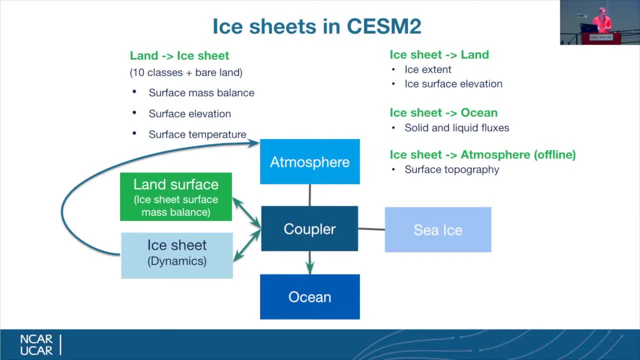 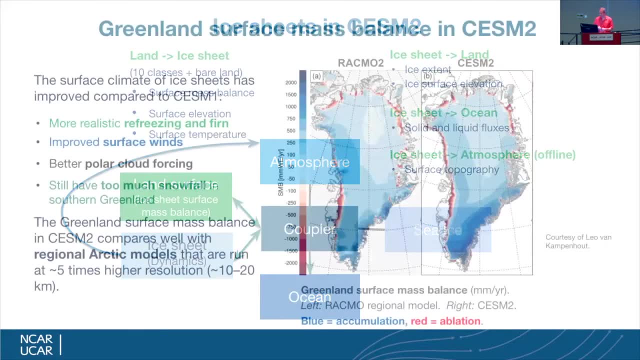 model, reset the atmospheric topography and restart it again every 10 years or so. So that's what we've done in simulations of longer than a few years. So one of the things we were excited about for CSM2 was we had a better Greenland mass balance. 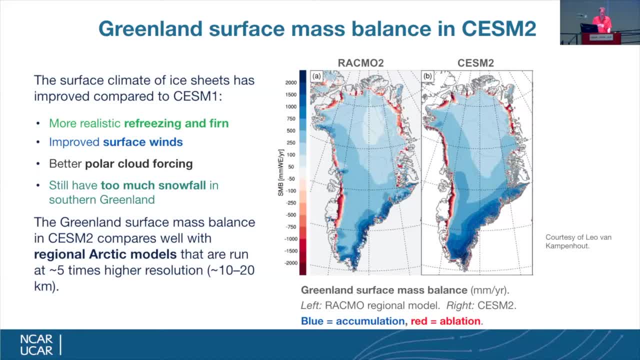 and there were some improvements in the treatment of snow and fern, which is snow, that's in transition between snow and ice. better winds, better polar clouds. We do still have, for Greenland, a significant bias, which is illustrated in the pictures on the left, where, because of 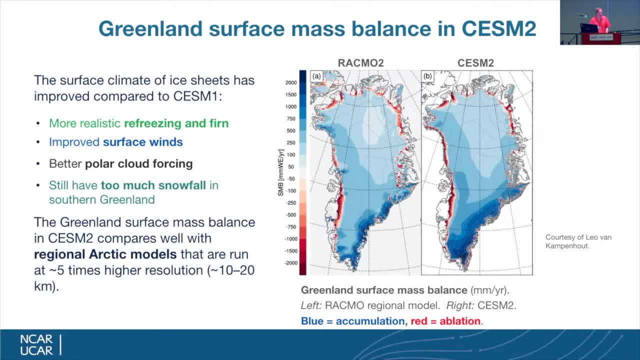 the relatively coarse one-degree model resolution. the topography in the south of Greenland is not well represented, And so we have too much snowfall. then, instead of being concentrated along the south southeast coast, works its way in the interior and contributes to the 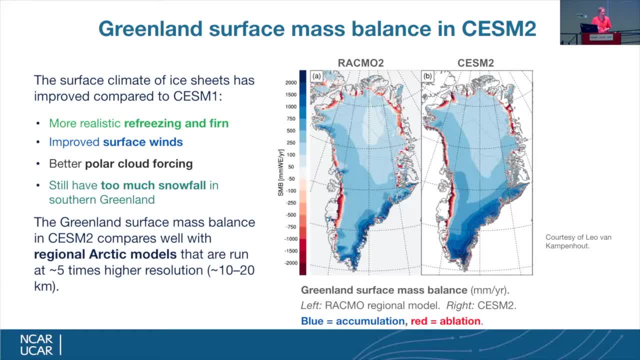 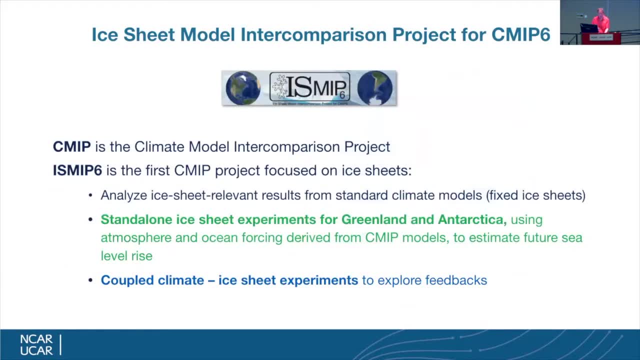 building up the ice sheet, So that's a bias that we're trying to improve by improved resolution or other means. One of the motivations for making these changes was to participate in something called the Ice Sheet Model Intercomparison Project for CMIP6, or ISMIP6,, which was the first ice sheet component of CMIP. 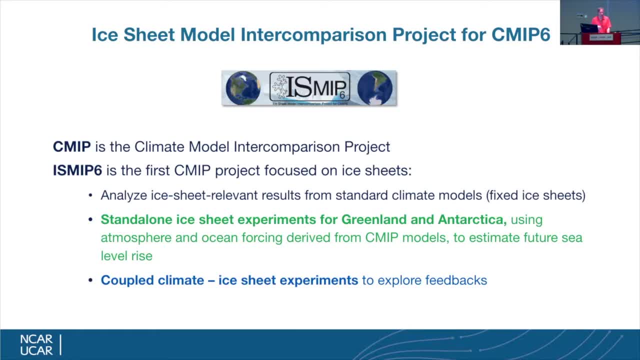 And it had several parts, including just analyzing ice sheet relevant fields from all models, but also doing standalone ice sheet model experiments in which the atmosphere and ocean forcing was derived from a whole suite of global climate models, And also the first stages of experimenting with ice sheets interacting with the climate, which at this point, only a few models can do. 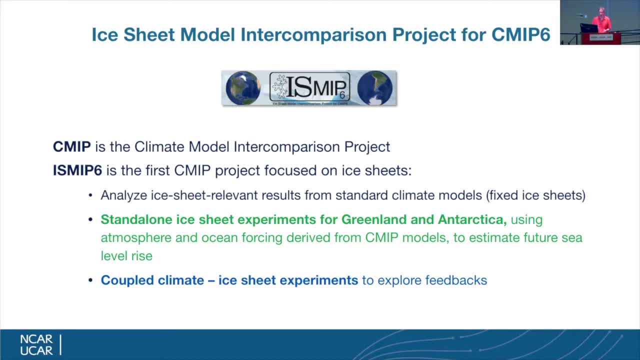 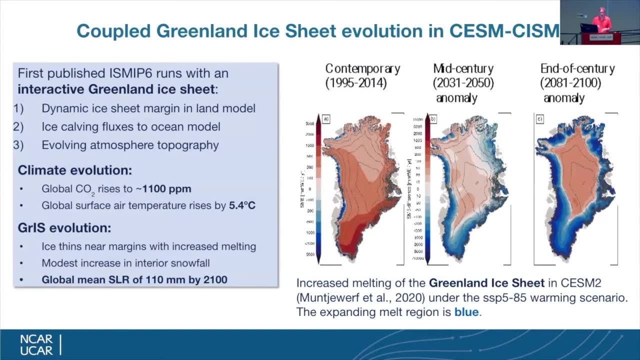 with CSM being one of those models. But when you have the interactive coupling, of course, then you can explore feedbacks. So CSM was the first. It was the first model to have published papers describing runs at relatively high global resolution of about a degree and an interactive Greenland ice sheet. 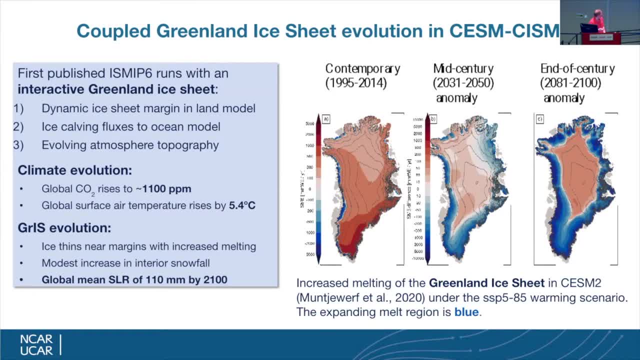 We ran the model in different configurations. This is the SSP585 high emission configuration. You can see from the figures on the right that the blue region where you have a negative surface mass balance and melting, expands enormously as CO2 increases to above 1000 parts per second. 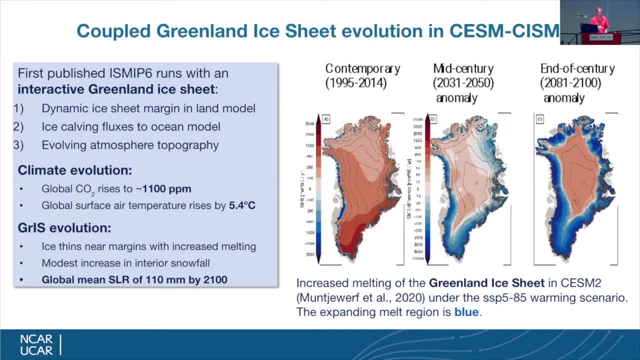 While we have big reductions of CO2 and CO3 in these simulations, down to about 300 parts per million, And this leads to about a hundred millimeters of sea level rise over the course of the 21st century. in the simulations, However, we did not find a significant feedback effect in the sense that, while the AMOC weakens in the simulations, 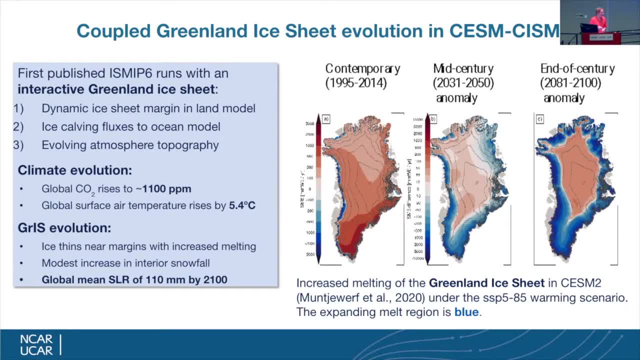 whether or not you have an interactive Greenland weakens by about the same amount. So at least at this level of sea level rise, the Greenland feedbacks on the ocean are not as big as people have expected, So it's difficult to really say right now. 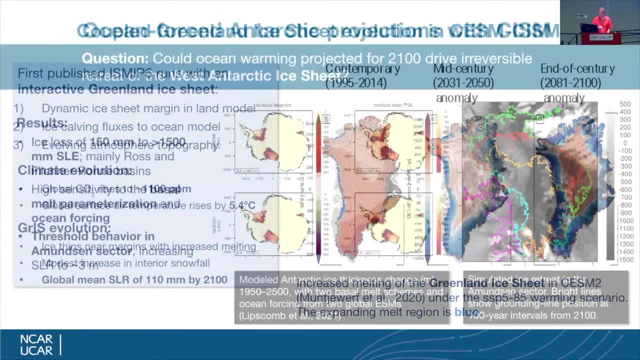 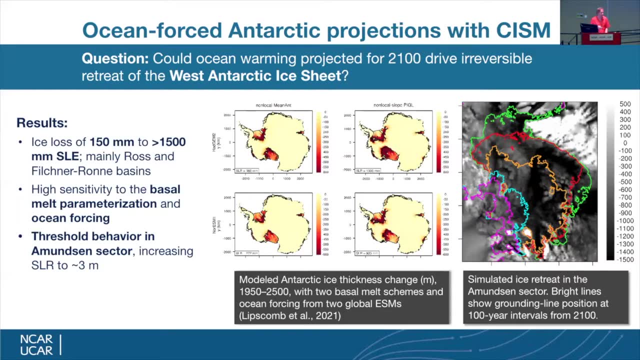 I'm really curious: is there any you can tell us how you pull it together have been concerned about? We didn't have a couple of Antarctica, but we did, with CISM, a lot of standalone experiments with the Antarctic ice sheet, And one thing we found is that the response. 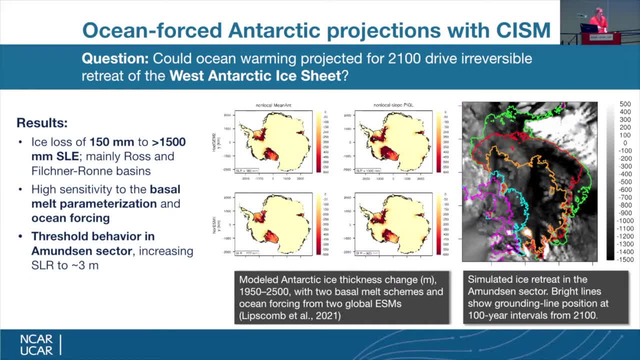 of Antarctica to warming of a few degrees depends a lot on what the ocean forcing is and what the physics parameters are in the ice sheet model. So we found sea level rise for Antarctica over the next few centuries of anywhere from up, say, 150 millimeters to upwards of 1.5 meters. 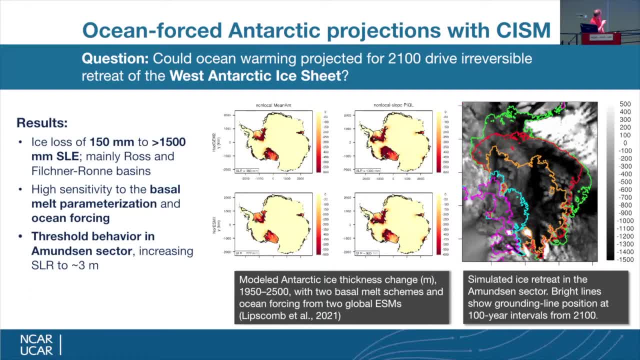 Most of the sea level rise is in the regions that are shaded red in the middle panels: in the Fils-Norani ice shelf to the upper end and the Ross ice shelf to the lower end, And the region where most ice sheet retreats happen today in the Thwaites and Pine Island. 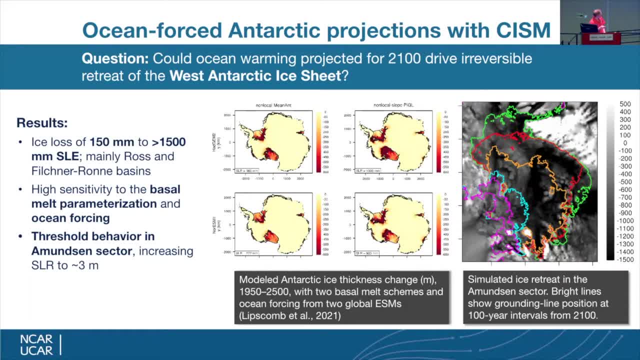 glaciers. that region is illustrated on the right And what we found there is that, under relatively modest measurements, the ice sheet retreats are shaded red in the middle panels. There's almost no change, but you reach a threshold at about one and a half or two degrees. 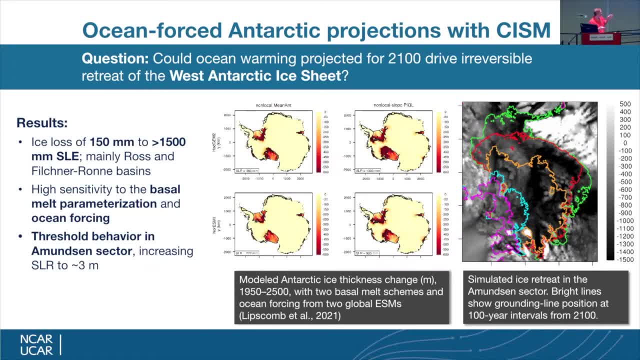 of warming and then you drive unstable retreat through this basin, which is the darker region of the plot, And that adds another meter more of sea level rise. So obviously something we need to do better is understand the thresholds for instability of the Thwaites Pine Island region. 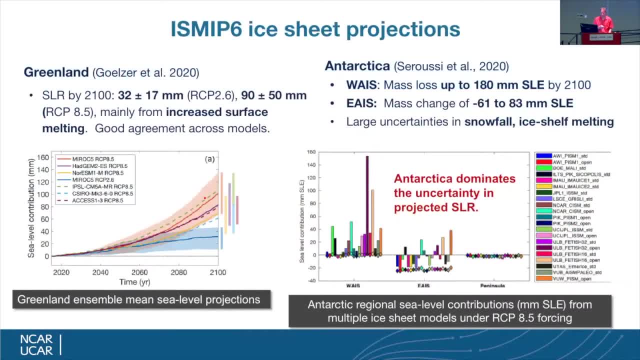 or the Amundsen Sea Embayment. So CSM and CISM were just one of many groups that contributed to this And we found that there was a lot of change And we found that there was a lot of 1206.. And if you put everything together, you find a fairly consistent picture for Greenland. 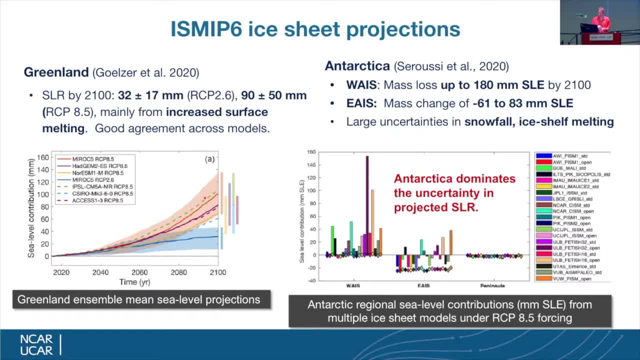 where you have under the high emission scenario is about 10 centimeters of sea level rise between now and 2100, with most of that being from increased surface melting For Antarctica. however, the models are all over the place, with estimates from ways ranging from: 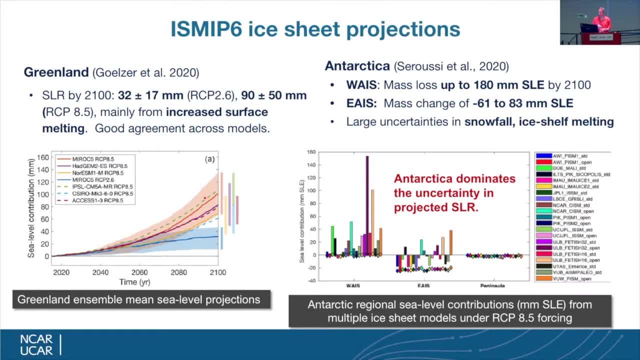 anywhere to just very small, to about 20 centimeters or 20 centimeters, And so we have a lot of, or 200 millimeters of sea level rise by 2100.. And then East Antarctica being all over the place, because in some models snowfall increases enough. 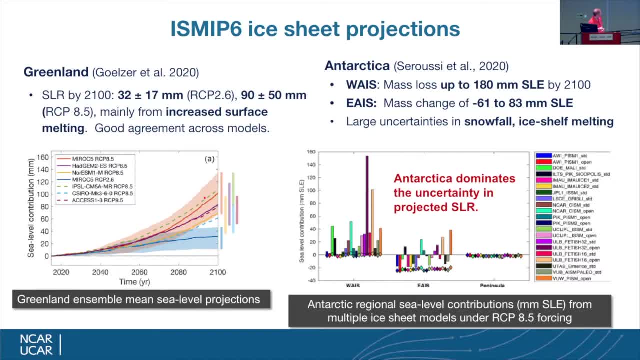 in East Antarctica to balance most of the melting And in some cases, to balance most of the melting in the West Antarctica as well. So in that you have projections of anywhere from almost zero to several tens of centimeters of sea level rise. So this is obviously a place that the models need. 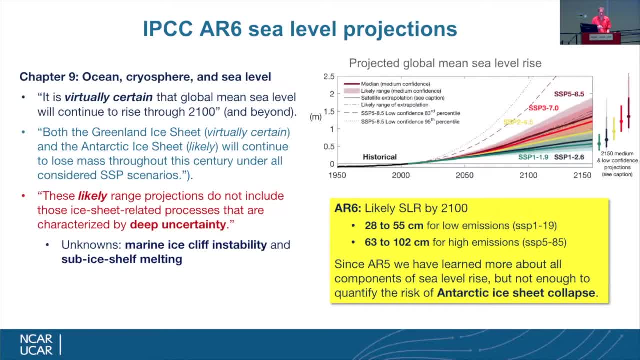 to do better to make meaningful sea level projections. If you look at the bottom line sea level numbers for AR6 shown in the yellow box for high emission scenarios, you're looking at about 60 to 100 centimeters of sea level rise from all sources. 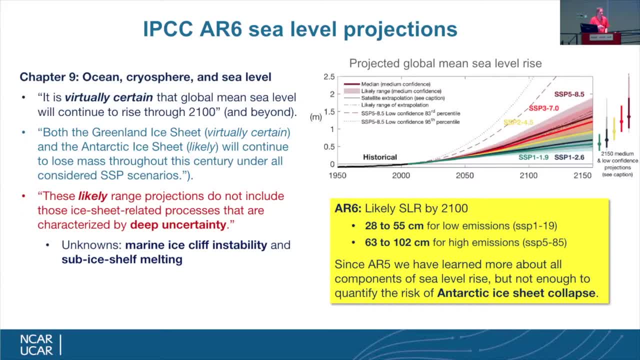 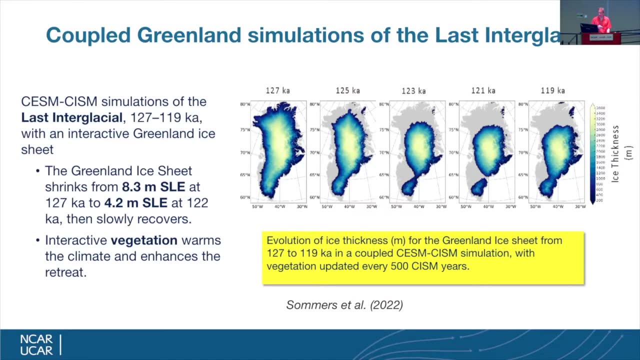 including land, ice and ocean thermal expansion, But with some big caveats about those numbers being could be significantly different if there were Antarctic ice sheet collapse. So in the last few minutes I'd just like to talk about some more recent work that's been done during the model. 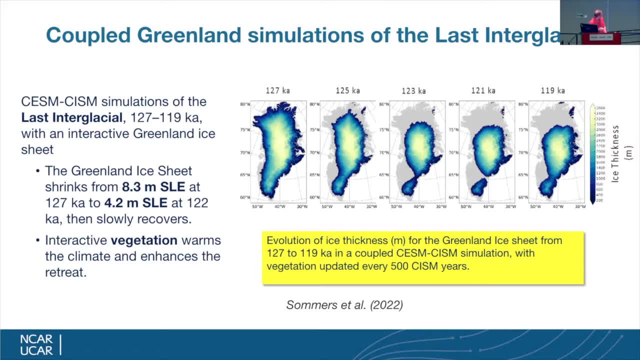 This is work by Aaliyah Summers, et al Aaliyah was a postdoc here a couple of years ago. We did simulations of the Lasterner glacial period from 127,000 to about 119,000 years ago And we did asynchronous coupling of the ice sheet. 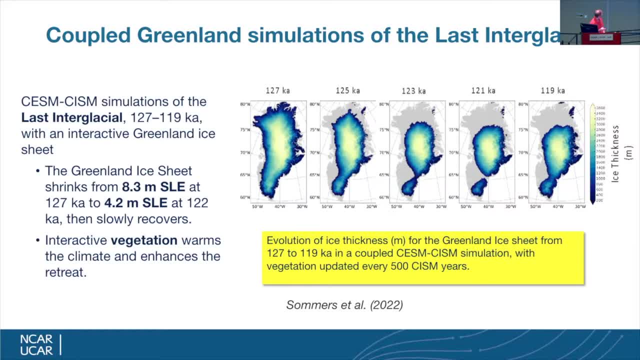 and so that we could afford to run an 8,000 year simulation, CSM. you can see, starting from an ice sheet that's close to present day, you lose about half of it by about 121,000 years ago And at that point the orbital conditions are such that you no longer 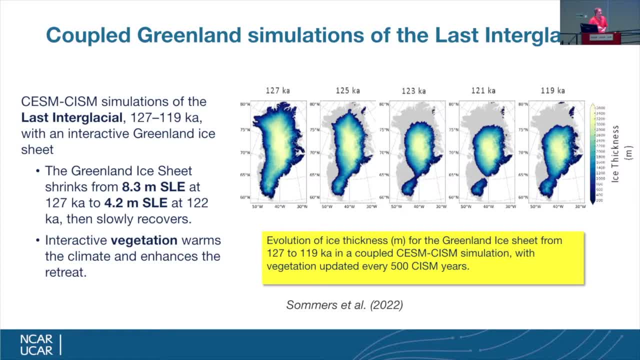 have as much melting and the ice sheet slowly recovers. A key finding of these simulations is that it depends a lot what the vegetation does. If you don't have interactive vegetation, then the albedos and local climate of Greenland and upstream in Canada are not as warm and you don't 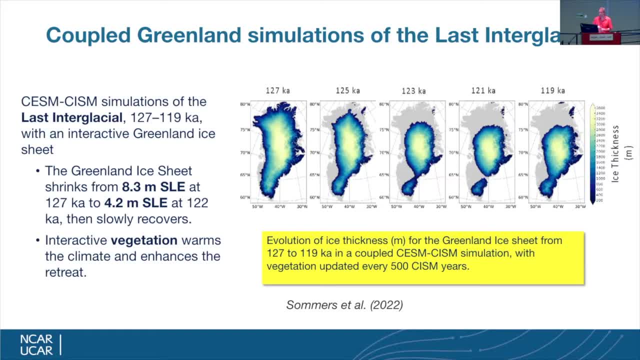 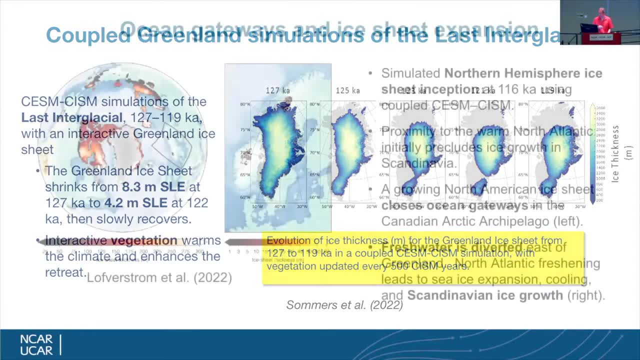 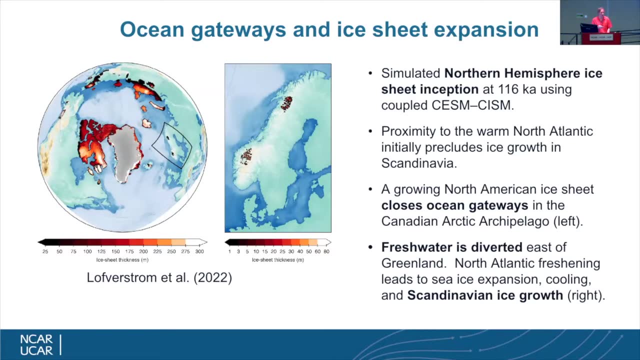 have nearly as much ice sheet retreat, So this points to the importance of having dynamic vegetation as part of the whole picture of what ice sheets are doing during warm periods. We also simulated the ice sheet inception that occurred around 116,000 years ago as we were coming out of the last interglacial And, encouragingly, CSM is able to predict. 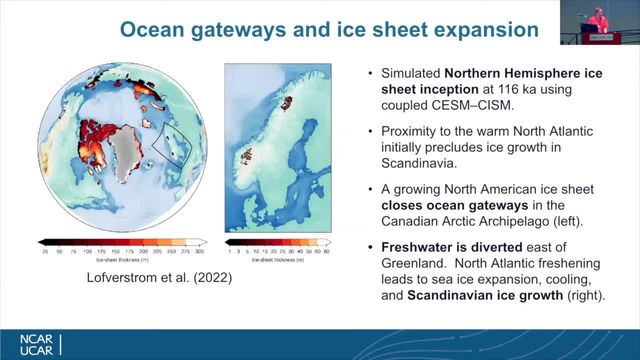 with pretty good accuracy where ice is likely to form as the climate cools. So, in particular, the ice sheet is likely to form as the climate cools, In particular in the Canadian archipelago and around the margins of Greenland. probably too much ice in Siberia, which is a common problem in models of trying to simulate. 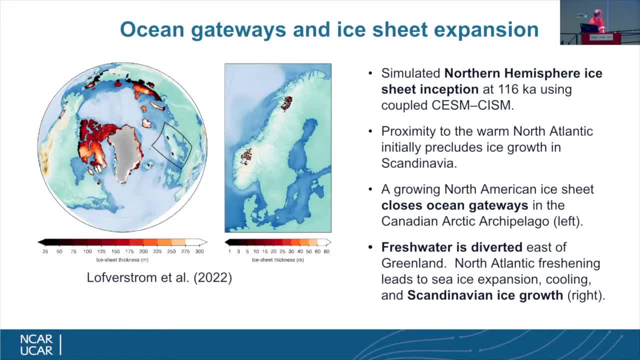 inception. Interestingly, we found not enough simulation, not enough ice forming in Scandinavia, where it's known that there was a small ice sheet. But it turns out that closing ocean gateways in the Canadian archipelago and redistributing the ocean circulation changes the regional climate. 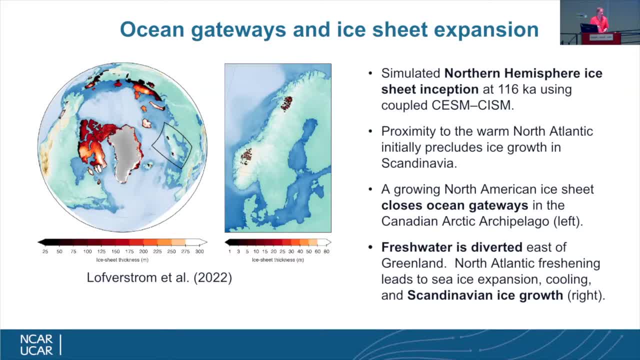 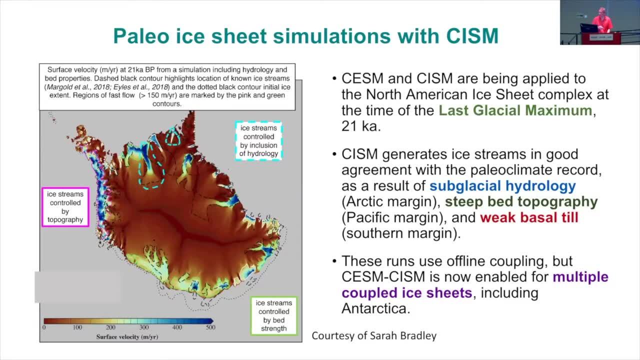 enough that you actually do start growing ice in Scandinavia, as the paleo climate record suggests did happen. Moving up in time some more, going to the last glacial maximum, about 21,000 years ago, you had a huge ice sheet covering what's now Canada and the northern US. 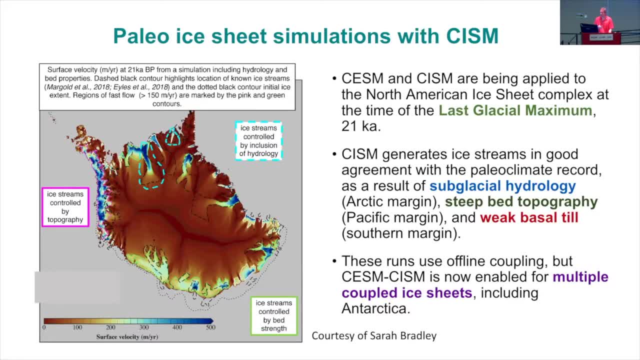 And these were the first experiments to use a new model of subglacial hydrology that we developed, And an interesting thing here is that you have paleo records showing where there were ice streams 21,000 years ago in this huge ice sheet, And so of course you wonder: does your model just? 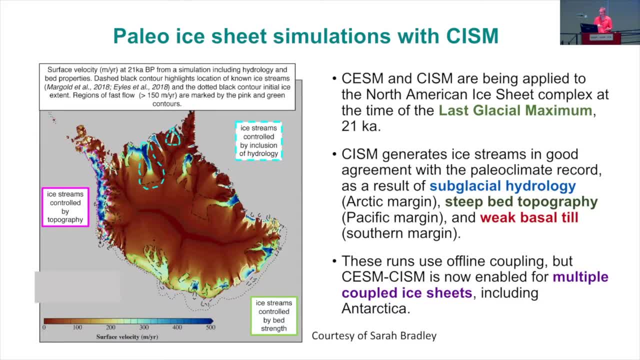 generate those as observed or not, And actually the model does pretty well at putting ice streams where we think there were ice streams. These are the fast-flowing blue regions in the bottom left And interestingly, the ice sheets form in different parts of the ice sheet for different reasons. 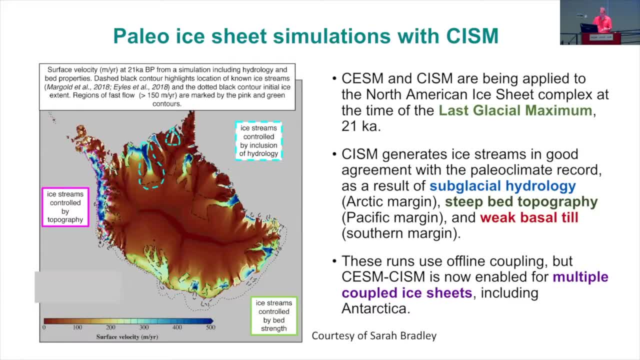 Some combination of the subglacial hydrology that makes the ice flow faster because there's water there, making the making the bed more slippery, or steep topography, or the southern margin weak, basal, till that allows the ice front to advance into what's now the 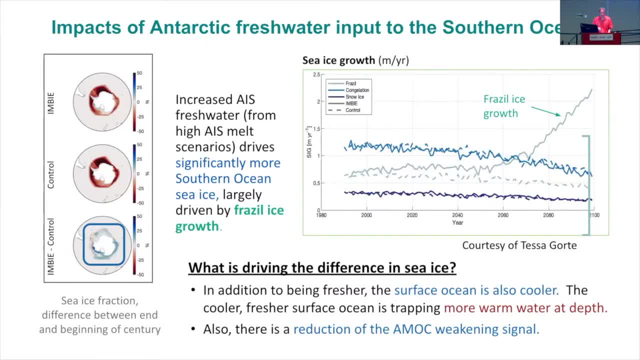 northern US. We're also beginning to explore more of the effects of changing ice sheets on the rest of the Earth's climate. This was a set of simulations done recently where, using a high ice sheet retreat scenario, we were able to see that the ice sheet retreats were going to be. 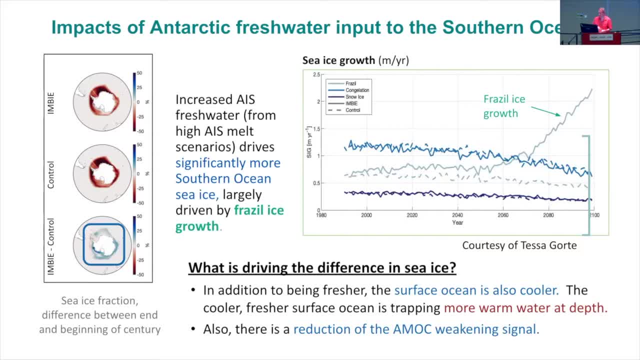 in the southern ocean and then see what happens. And what happens is you have a lot more southern ocean sea ice, with the main mechanism being that the melt water not only is fresh, but is cooler and traps more warm water below the surface and allows sea ice to expand more, And it also reduces 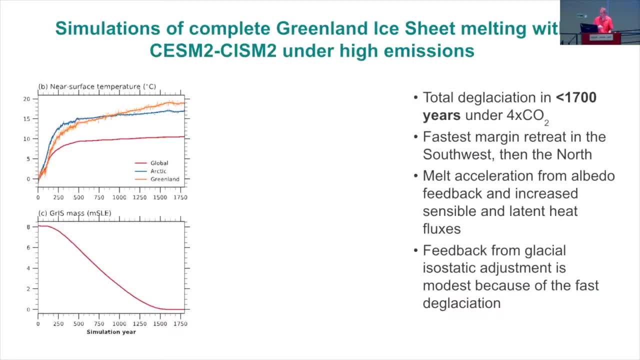 the weakening of the AMOC, the overturning circulation which is otherwise seen in the simulation And, um sorry, there's supposed to be a plot in the middle showing Greenland. but the bottom line is when you continue a high emission scenario with quadruple CO2, and just keep it going out for 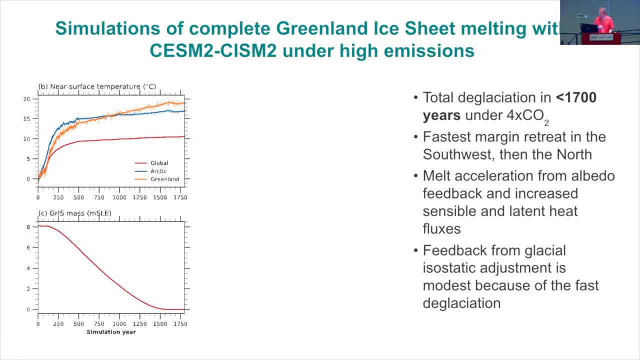 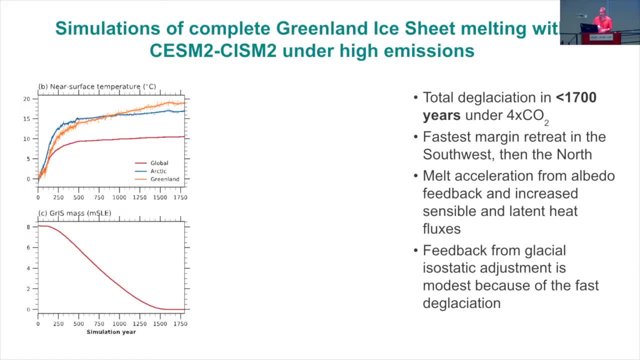 So that is where you end up with that point of of no return and where the Greenland ice sheet is inevitably going to be lost in a period of you lose most of it in the first 1,000 years or so. But the good news is if, in the case of Greenland, if you were able to lower the temperatures. 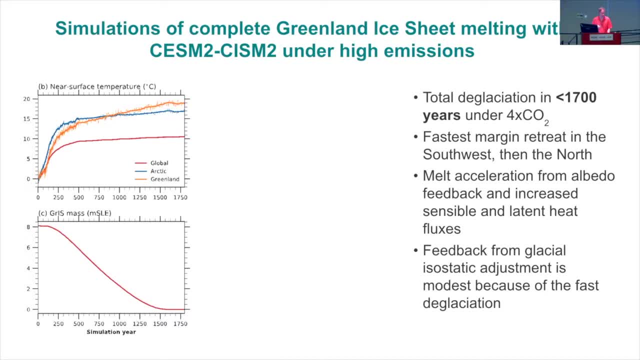 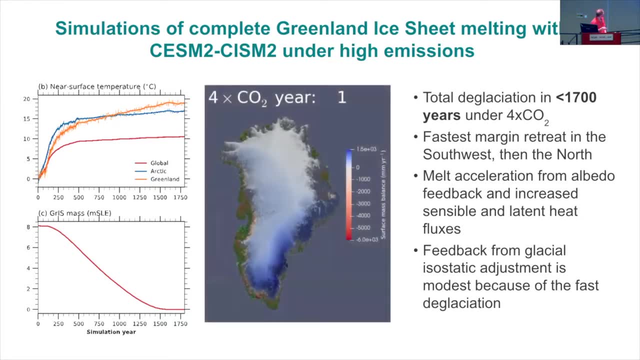 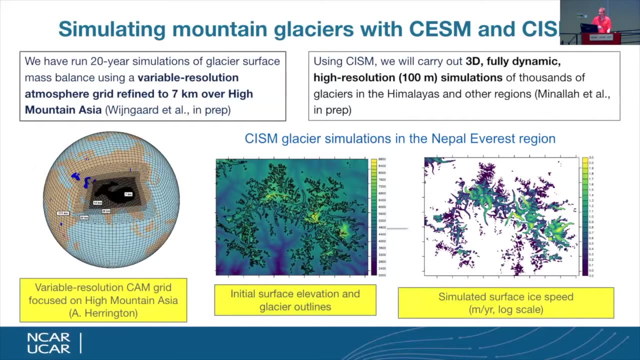 most of the ice sheet does grow back until you get to a point where most of the ice sheet is is gone. Ah, there it is. Well, I'll move along. Another new initiative is to not just simulate ice sheets, but also to simulate. 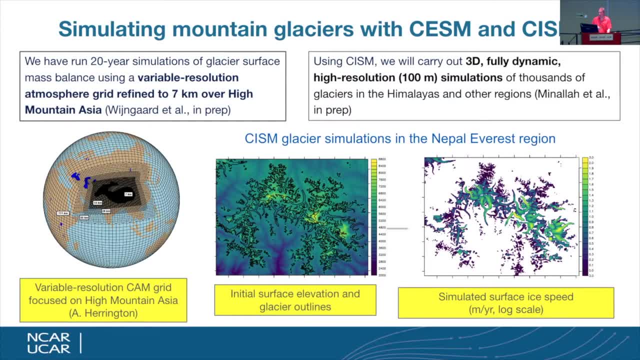 mountain glaciers. We have an ice sheet model which we've just recently started using as a model for glaciers as well. The physics is fundamentally the same whether you have an entire ice sheet or a smaller complex of glaciers. The main challenge is just in the sheer number of 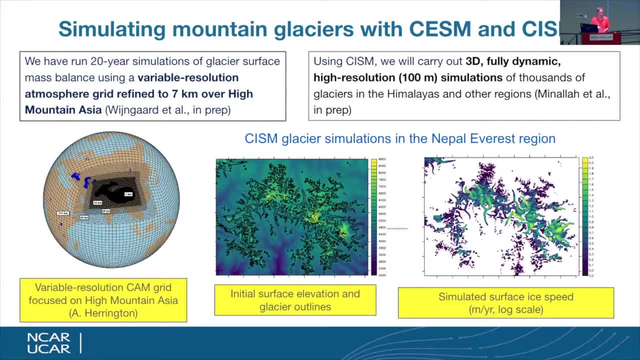 glaciers and the fact that they're much smaller and need to be resolved with much higher resolution. Our typical resolution for ice sheets is around a four-kilometer grid, but for glaciers we need around a 100-meter grid, so a many times increase in computational. 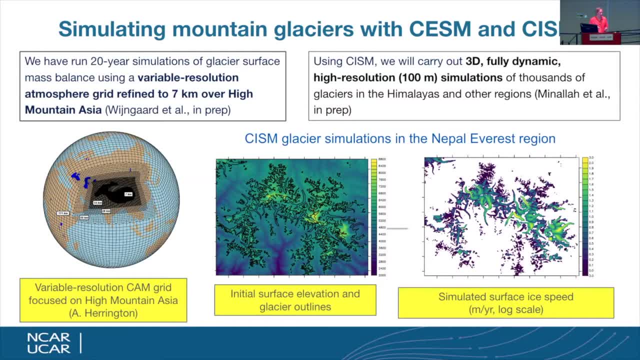 cost per unit area. Fortunately, the area of mountain glaciers is not that big compared to ice sheets, so it does look like it's going to be computationally feasible to simulate large numbers of glaciers. The plots shown here are for a pilot case where we're just looking at glaciers in the Nepal-Himalayas. 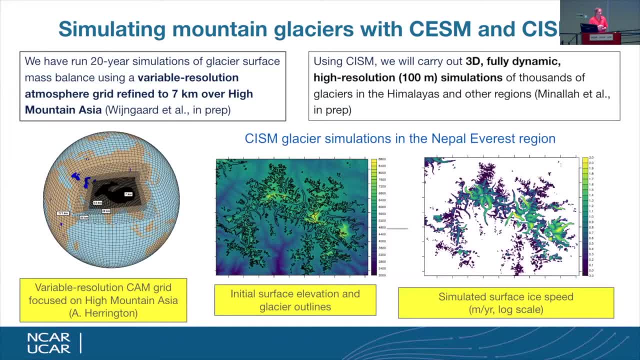 this being the Everest region. By doing some tuning to make the surface mass balance of glaciers consistent with observations, we can simulate glacier thickness and glacier speeds that are in good agreement with observations. A related project you may have heard earlier in the week about variable resolution, CSM- where, with the spectral element, 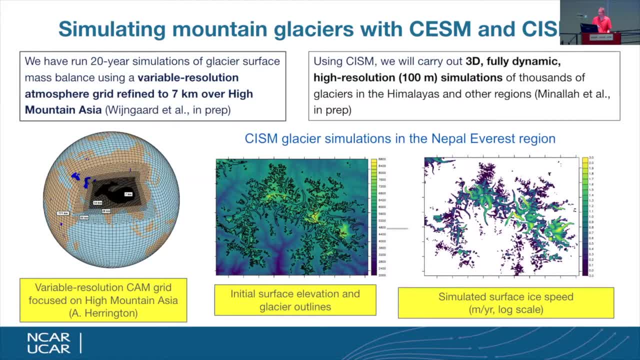 the chemical core of the atmosphere. we can selectively refine regions. So one of the selectively refined regions is the grid shown on the left, where you have refinement of as fine as seven kilometers over high mountain Asia. One of the goals of these simulations is to 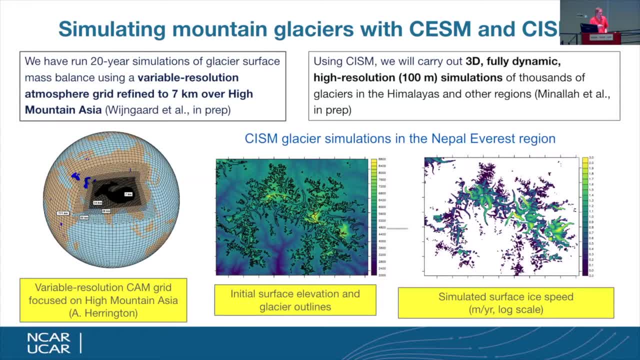 accurately simulate the surface mass balance of glaciers so as to predict how the surface mass balance will change in the future. At present, the surface mass balance is still more negative than observed, so we're trying to simulate an increased surface mass balance, Even though it's not exactly. говоритon that it's still an extreme problem. we have to be very careful of that, because when we're trying to simulate an extreme problem, we have to be very careful about the changes in the situation. So we have to be very careful to anticipate and interpret the changes in the future. So, for example, 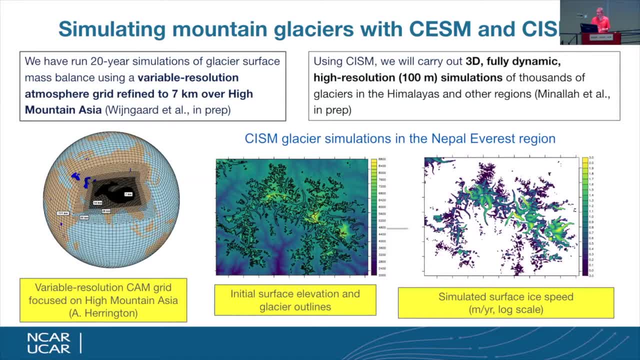 if we're trying to estimate an extreme problem, we have to be very careful of the changes in the situation, trying to sort out what are the scale-dependent things in the model that may need to be changed in order to have a more accurate surface mass balance simulation. 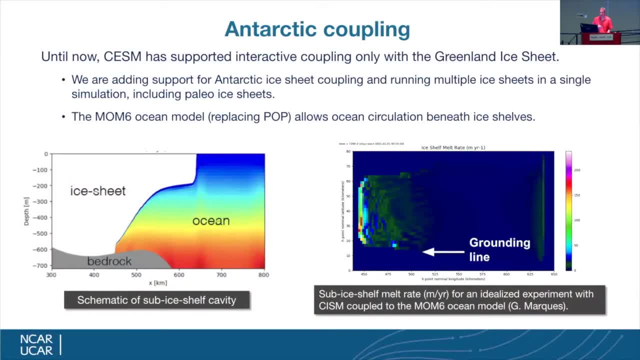 And also we are now supporting coupling interactively with Antarctica. This involves having an ocean model, MOB6, the new ocean component that will circulate under ice sheets and can change its shape. The shape of the ice-ocean boundary can change as the ice sheet. 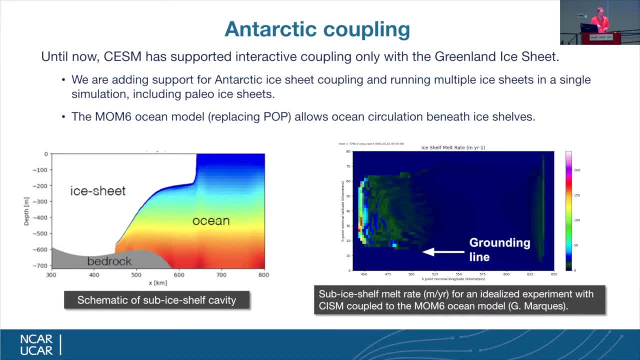 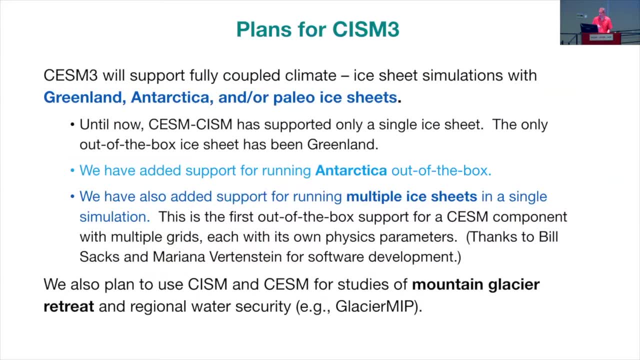 melts And we now have most of the technical software coupling parts in the model to do this and we're just beginning to test the coupling. So for CSM3, we want to support interactive coupling not just with Greenland, as in CSM2, but also with Antarctica and also with paleo-ice sheets. 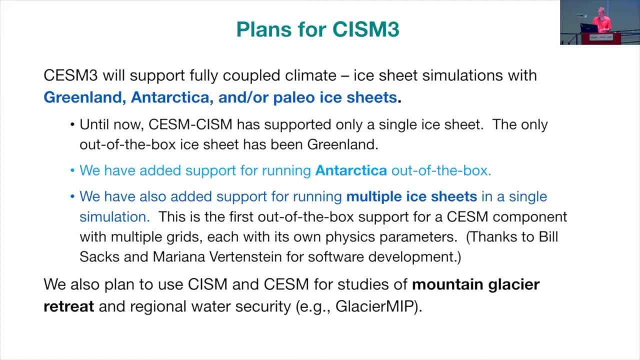 which we now have the technical ability to do on developmental branches and are just starting to test and make sure that it all works, And also in CSM3, you'll see that we're starting to test and make sure that it all works And also in CSM3,. 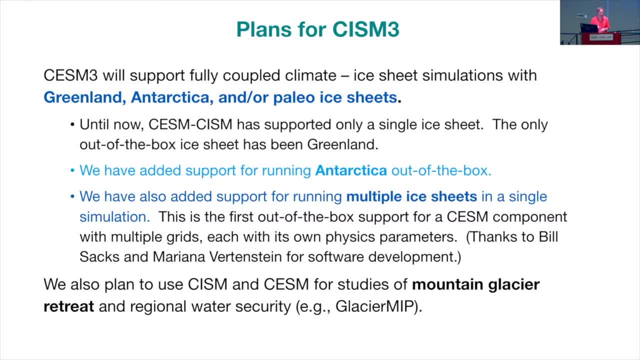 you'll see that we're starting to test and make sure that it all works, And also in CSM3, you'll be able to run with as many ice sheet domains as you'd like at one time. Typically, this would be Antarctica and Greenland, or Antarctica and a Northern Hemisphere- paleo-ice. 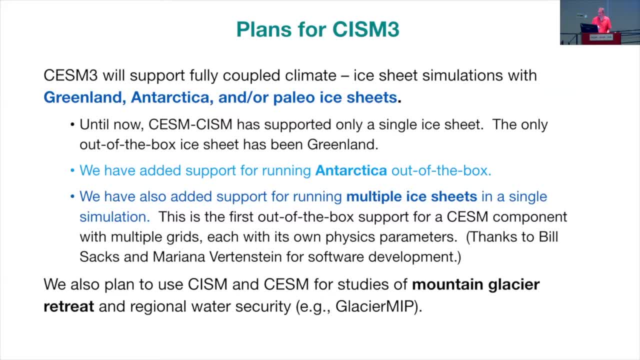 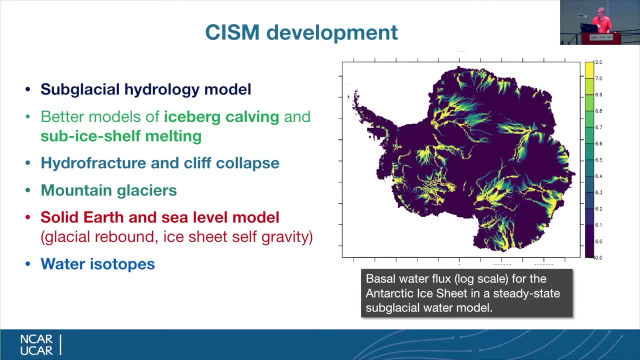 sheet And, as I said, we're also planning to get into the realm of mountain glacier studies and contribute to a project called GlacierMIP, which is like ISMIP6, but for the world's glaciers, And there's always model development to do. For CSM3, there's a number of physical components. 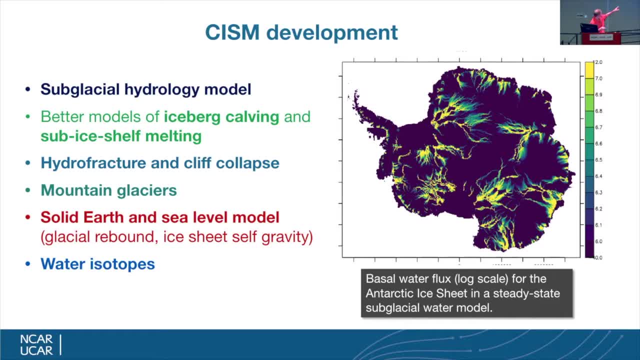 we're trying to improve For CSM3, there's a number of physical components we're trying to improve For CSM3, there's a number of physical components. we're trying to improve Subglacial hydrology, which is illustrated on the right, where you have basal water flow down the hydraulic gradient of. 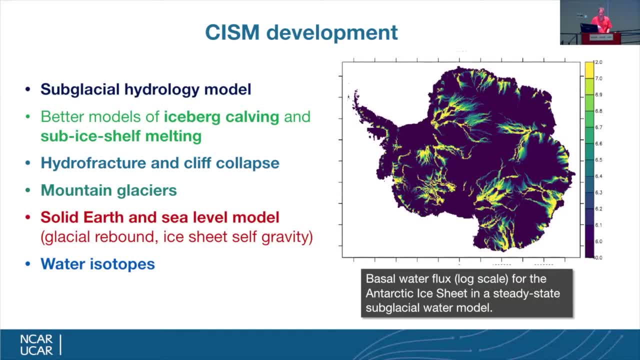 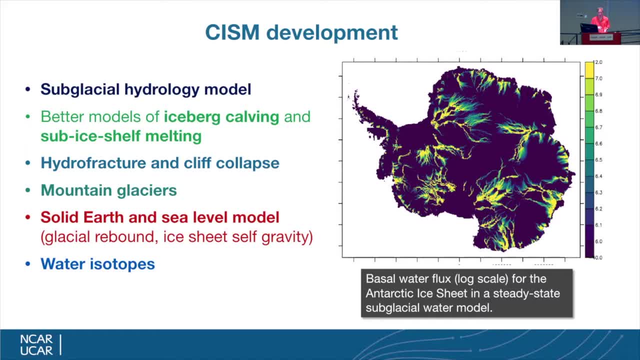 So you can include feedback such as, for example, as an ice sheet loses mass, the load on the earth is less, And so the earth can rebound, And that's a potential negative feedback on ice retreat, as is the self-gravity effect that I mentioned earlier. 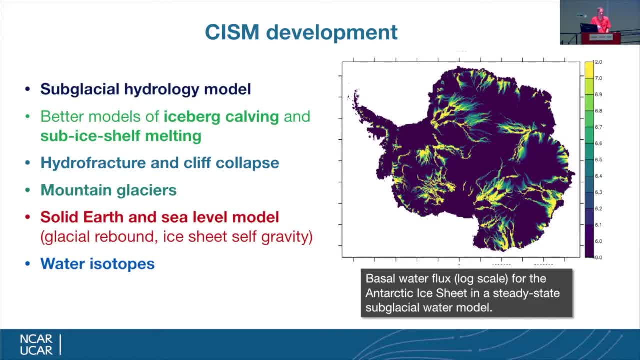 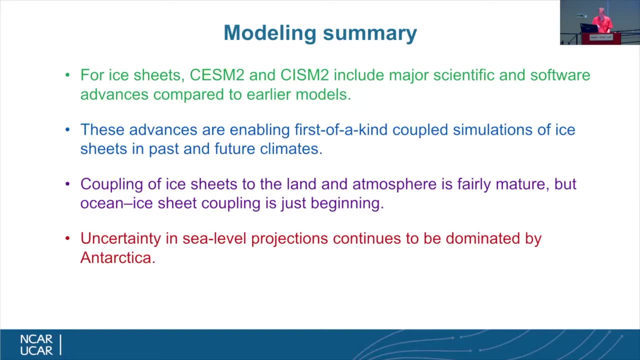 And the paleo folks are very interested in having water isotopes in the model so that we can track, for example, delta 018 through the earth system through the centuries, and land isotopes, of course is an important part of that. So just to summarize, CSM is pretty far along compared to 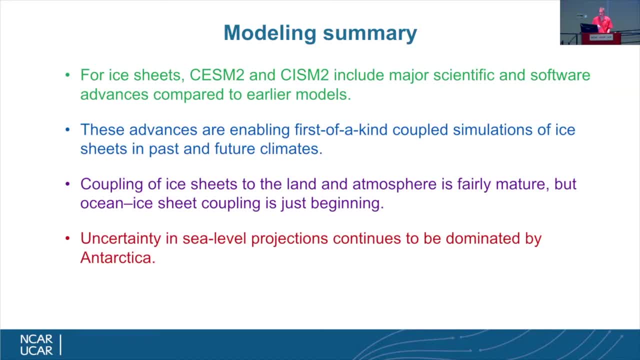 other Earth system models in having interactive ice sheets And we're now able to do the kinds of experiments that no one was able to do with the global Earth system model until very recently, And that's very exciting. And if any of you are interested in being part of these experiments, 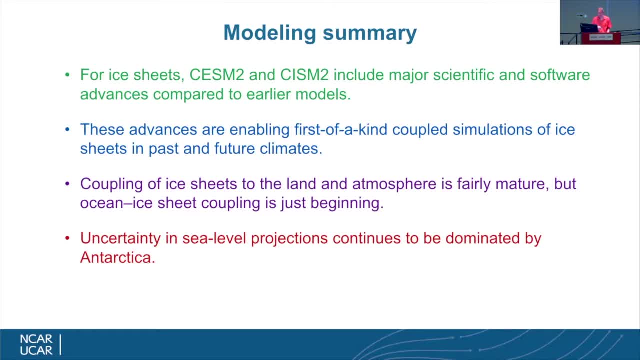 of course, let us know and we'd be glad to help you get started. The coupling to the ocean is still much harder and much less advanced than the coupling of land and atmosphere And the biggest problem for people concerned about sea level rise in the next few decades. 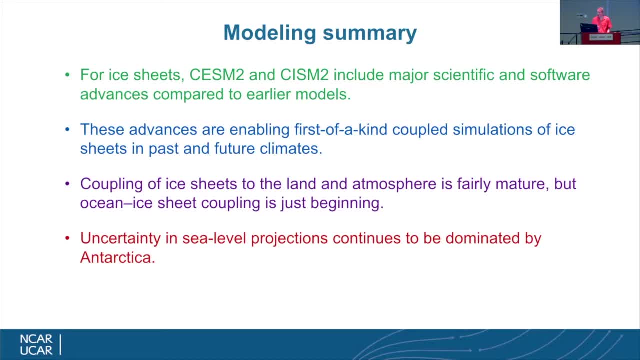 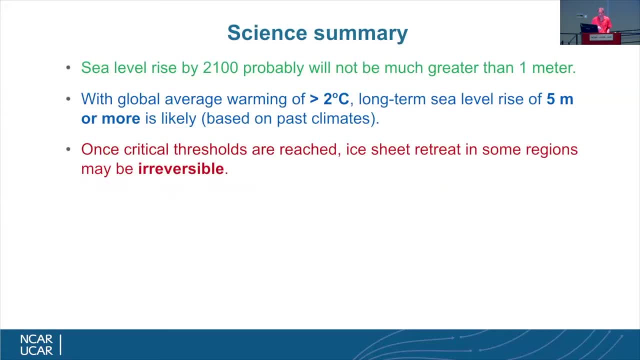 and centuries is: how do we model ice-ocean interactions around Antarctica and put better constraints on the Antarctic contribution to sea level? And scientifically, I would say that the most important thing is to be able to do this, And I think that's what we need to do, And I would say that sea level rise. well, obviously, sea level will keep. 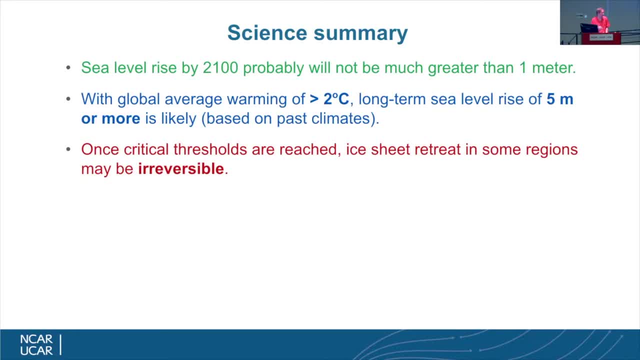 going up. It does seem unlikely that sea level rise would be greater than one meter in this century, Although for ice sheets this is an external process, And we're now entering a temperature range between one and two degrees where you have the potential of triggering larger. 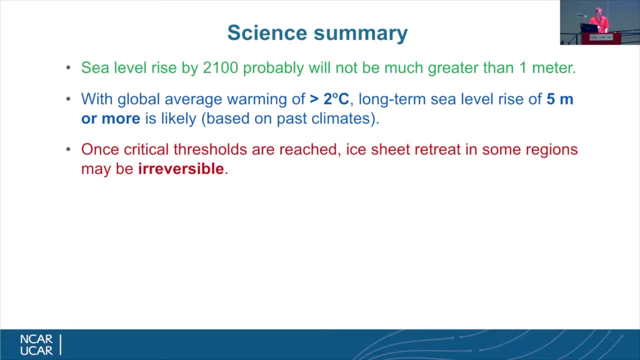 changes in ice sheet that could eventually lead to sea level rise of several meters or more. that may not be reversible, So that's still, of course, a major concern as we consider, for example, what trajectory we're going to be on, how close we'll come to the 1.5. 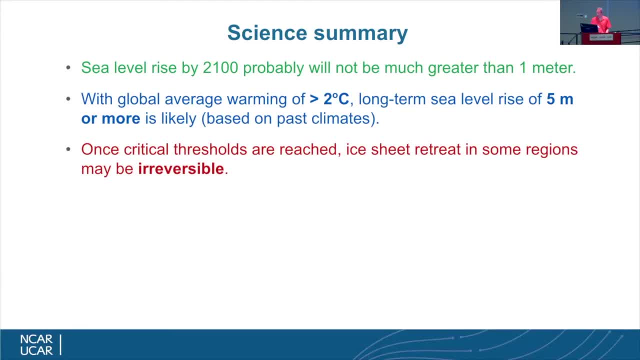 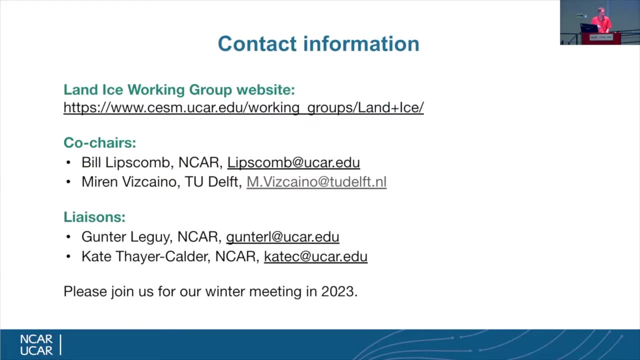 degree Paris target, or do we shoot past 1.5 to 2 degrees? And for ice sheets it potentially makes a major difference whether you stop at 1.5 or go on to two or more. So with that I'll wrap up. We're very glad to work with anybody who's interested in ice sheets. 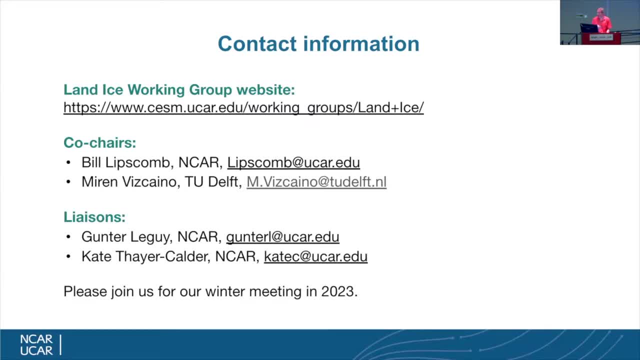 I'm one of the co-chairs of the Land Ice Working Group, along with Miriam Descano, who's at Delft In the Netherlands, And our liaisons are Gunter Lege and Kate Thayer Calder, who are not able. 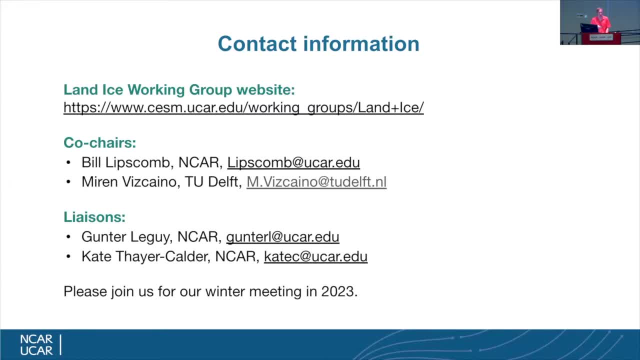 to be here today, but who are extremely helpful in helping people work with the model. And, of course, we have a winter meeting, like all the other working groups, and we'd love to see you, either virtually or in person, at our next winter meeting. So thanks. 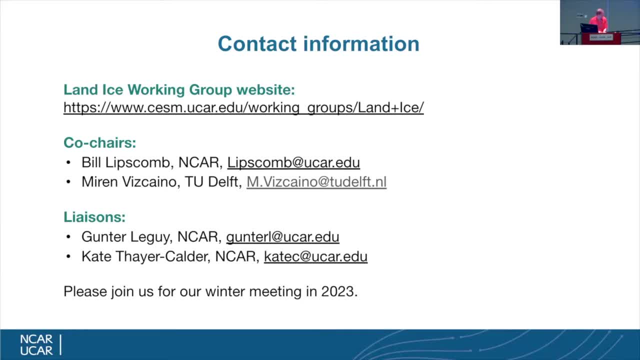 So thank you, Bill. That was really insightful. When you think you're modeling these ice sheets to have high resolution, 100 meters is really really high. Yeah, So it's fabulous looking at what's happening with the mountain glaciers as well as all the ice sheet work. So we have about 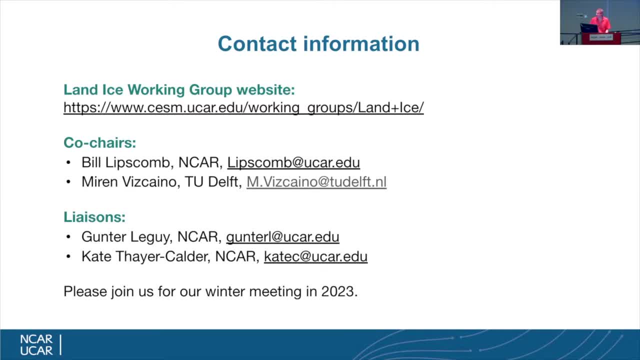 five minutes for questions. If people want to come to the microphones and address your question to Bill, that'd be great, Thank you, Hello. Thank you for your talk. I really enjoyed it. So the question I have is: so you mentioned that in parallel scene period the sea level is 5 to. 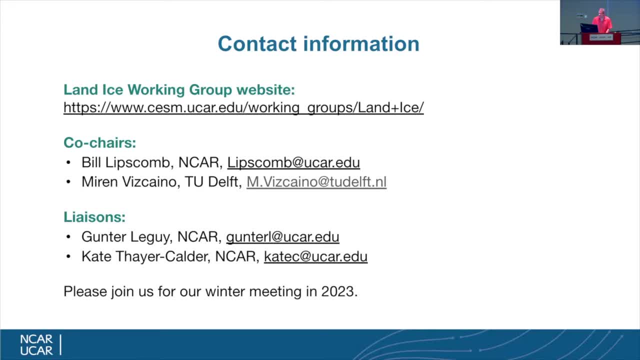 20 meters above. I was wondering just out of curiosity, because your ice model is kind of interact with land model, but the ocean grid cell is kind of fixed. So how would that affect our confidence about the paleoclimate simulations? Sorry, when you say the ocean grid cell, 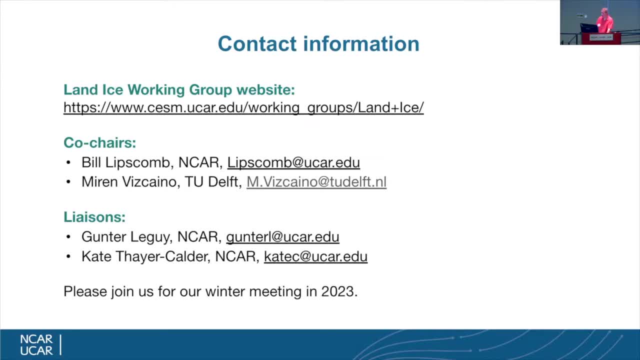 you mean the ocean horizontal grid? Yeah, Because the land-ocean boundary is fixed. you mean, Yeah, Yeah, It's a knotty problem. It's a knotty problem in terms of getting all the pieces to work together. Now, one of the great 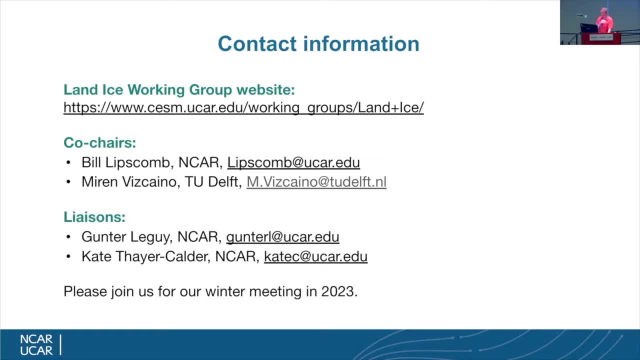 things about MOM is that, unlike POP, the older ocean model, MOM keeps track of the actual mass of the ocean And you can have ocean grid cells that have zero mass or any finite amount of mass. So with the ocean model, if you put more mass in the ocean, you actually will have ice moving up. 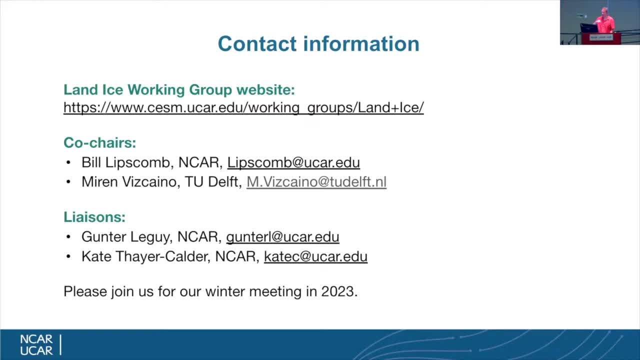 on shore, so that grid cells that were dry are now wet. So in that way you can have a lot of mass, And in that way it's not a problem for MOM6, because the model was designed to accommodate changes like that. What's trickier, I think, is the land model and the coupling. assume that if a 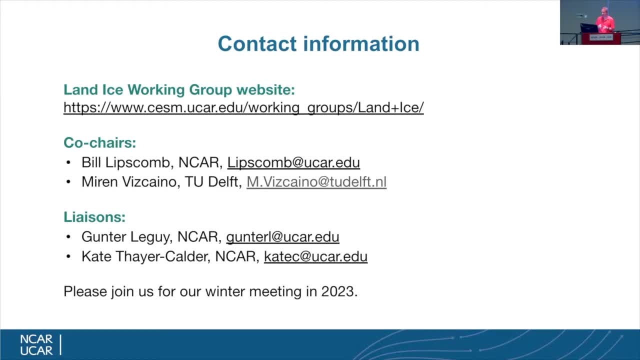 grid cell is land. once it's land, always. So, for example, if you have an ice shelf that's advancing, then as the ice shelf advances, it needs a surface mass balance which comes from the land model, And the land model as it's presently configured has no way of knowing that an ice shelf has moved. 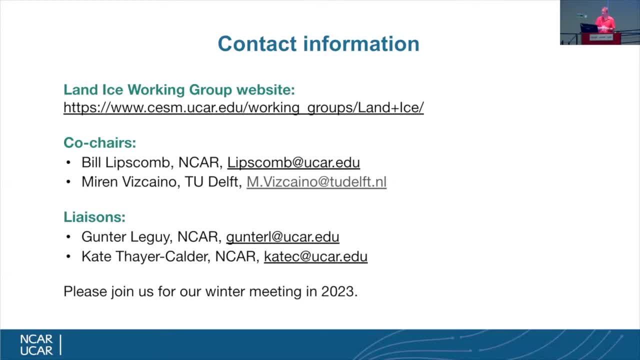 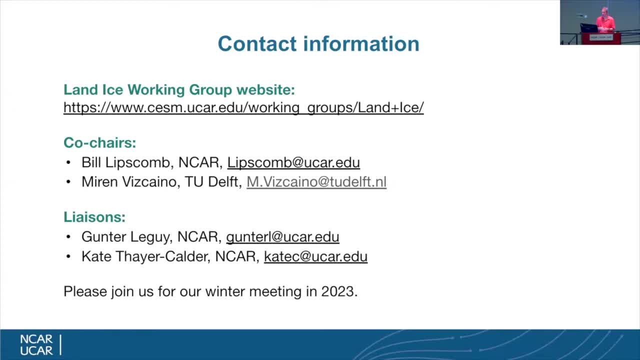 question. I think it's a great question. I think it's a great question. I think it's a great question on in the next year or so to enable that. Does that answer the question? Thank you, Yeah, I guess, just following up on that we were talking about how do we get the mass from land ice into? 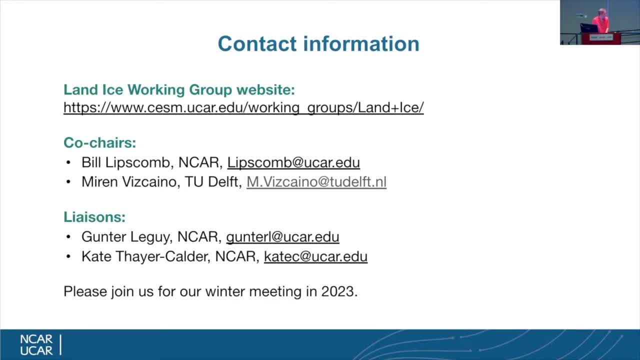 the sea ice when you carve So through the oceans and we're sort of saying, well, there's this snow capping parameterization that means we have a runoff of ice to the ocean which freshens the ocean and then that can refreeze the sea ice. but we don't really have this mechanism for. 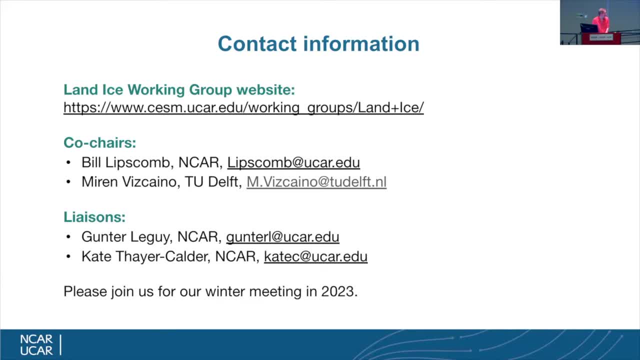 carving of icebergs and things like that. So that would be a good question. Another element of research, right, Yeah, I agree. Talk, I just had a question: what the current efforts are about the deglacial evolution of the glaciers and citizen and sort of especially characterizing like. 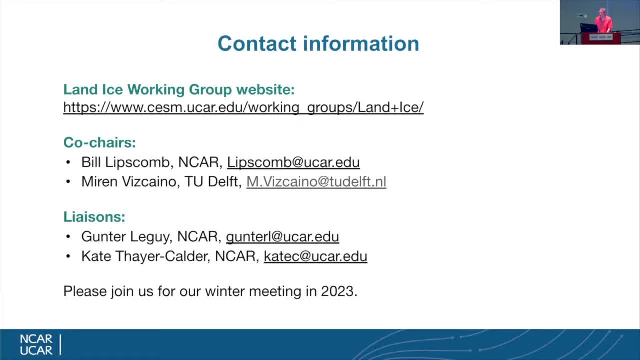 the millennial scale, like Heinrich stadiums and younger dry ice events, where you have the sort of these ice calving and potentially a mock disruption events, because I know currently that's not very well characterized. So what do we plan to do about that in the model? 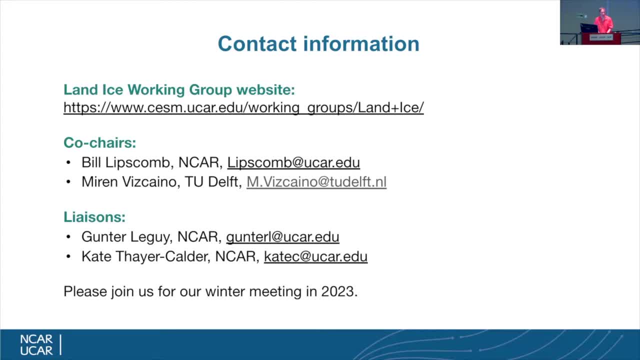 Well, right now I'm working with John and others on a proposal which would include expanding CSM capability so that we contribute, can simulate, for example, Heinrich events and put our allow armadas of icebergs to go to the ocean and move around and freshen the ocean. 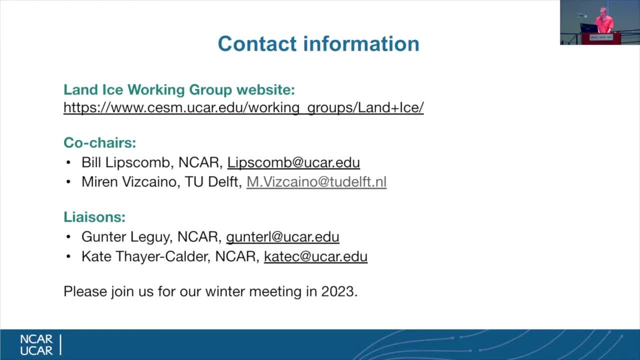 And we don't right now have the support to do that, But we're searching for the support to do that And with the, the resources, um, that is, that is high on our list. thank you, and yeah, that was sort of part of what dave bailey came up with yesterday in the discussion. 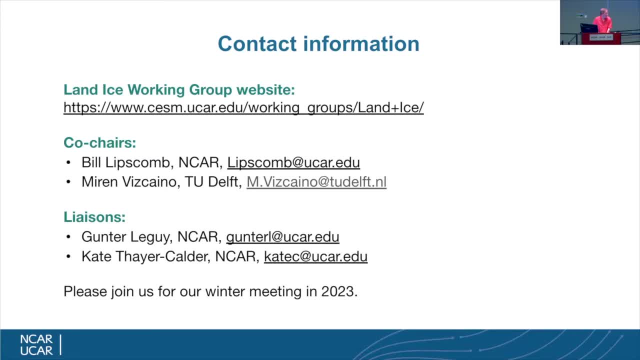 as well, was great like talking about the sea ice, land ice coupling. yeah, hi, thanks for that talk um that uh long-term simulation you did for the last interglacial. have you done something similar looking at the antarctic ice shelf and have you observed any like eastern antarctic melting in? 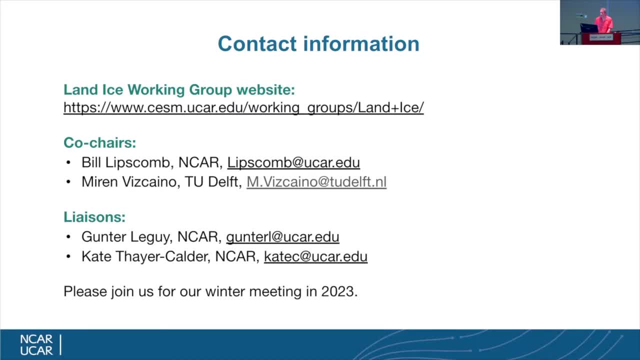 those scenarios, because i'm just thinking like the piacine is an equilibrated climate state. you mean like a multi-thousand year simulation. yes, with antarctica, um, not with csm. we, we can. we can do multi-thousand year simulations with a stand, with a standalone schism, standalone ice. 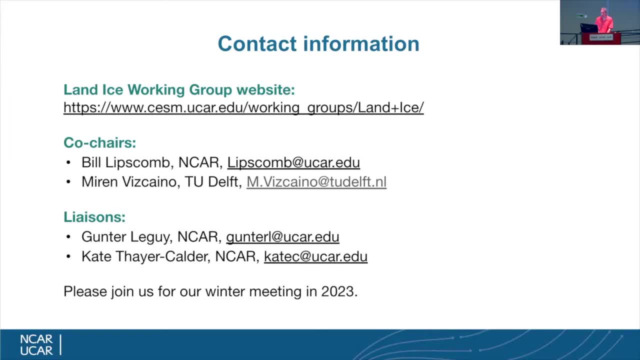 sheet, model um, and we do have a project ongoing where we're going to, where we're planning to do sort of partly coupled simulations involving the antarctic ice sheet and ocean forcing associated with the last interglacial. so sometime in the next one or two years those simulations should come out. 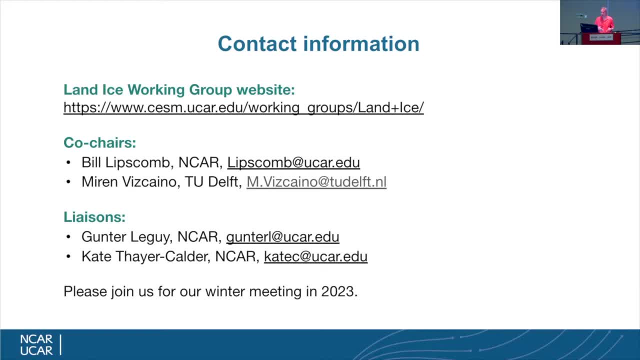 and so you'll have an ocean run. that's been say, it's been spun up or or advanced with orbital and co in greenhouse conditions corresponding to the last interglacial. and we're trying to understand, um, how antarctica advances under that changed forcing, because we 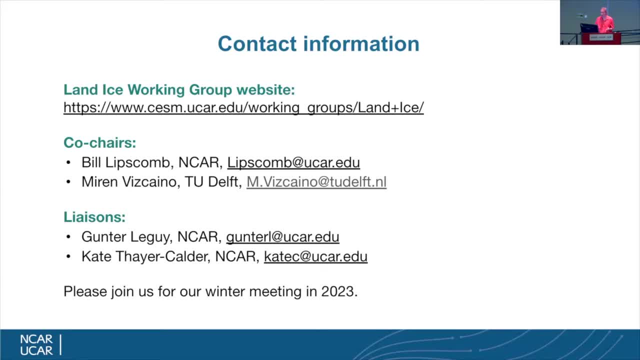 think that waste collapsed and lost several meters of sea level during the last interglacial, and so i guess that would be a step on the way to what you're talking about. where you have, i think what you're talking about, we have fully coupled csm, looking at antarctica on those time. 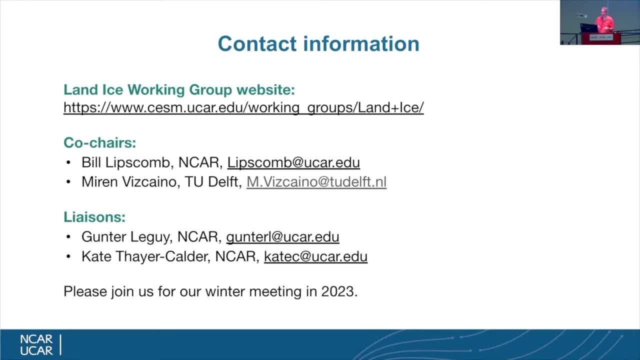 scales, so, um, so yeah, i guess we haven't done it, but we're obviously interested in- and you know, taking steps toward that. okay, is there anything on the same page that you're going to talk about? that is a fantastic time-span. we've got a lot of uh, maybe two or three hours to go. we've got a lot of time. 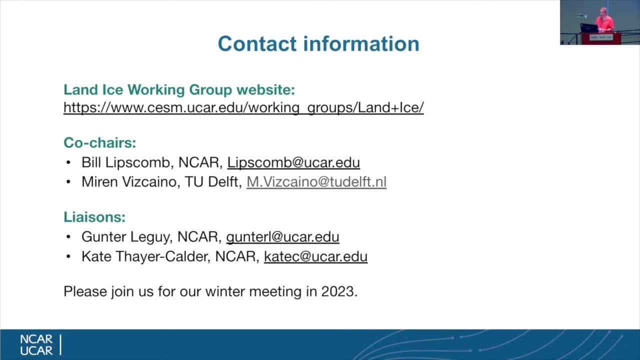 is that something you're interested in working on? yeah, well, i'm particularly interested in placing climate- ah okay, comparing that to future- future um climate change projections, yeah, and i'm just thinking like, if you have, if you're only running these future um ssp scenarios until 2100. 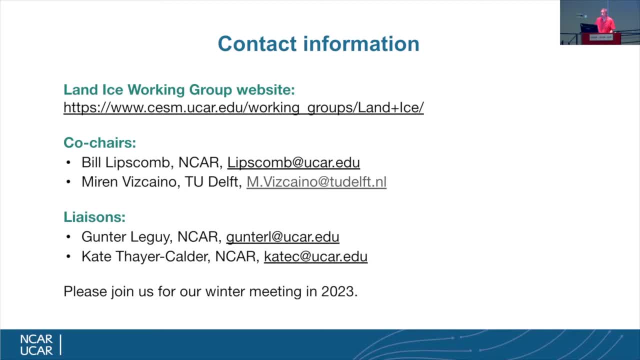 then maybe you don't. you're just not giving it enough time to observe east antarctic changes, perhaps? yeah for sure, and one of the things we're interested in is, in general, antarctica is not. you have to push antarctica pretty hard in terms of the ocean warming in order to get the 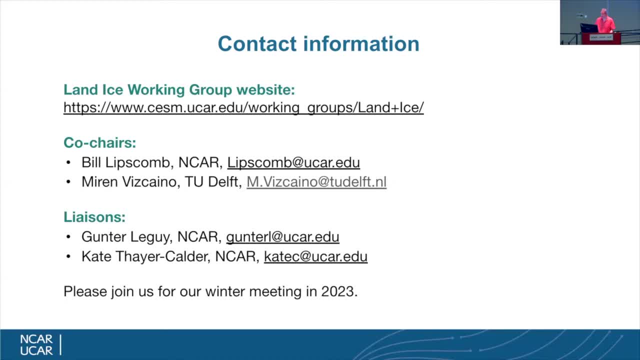 the ice sheet to lose many meters of sea level equivalent, and that might be because our ice sheet model is is too simple and lacking sensitivity in the physics, or it might be because we're missing coupled earth mechanisms, and one of the couple of models that we're looking at right now is the ice sheet model. 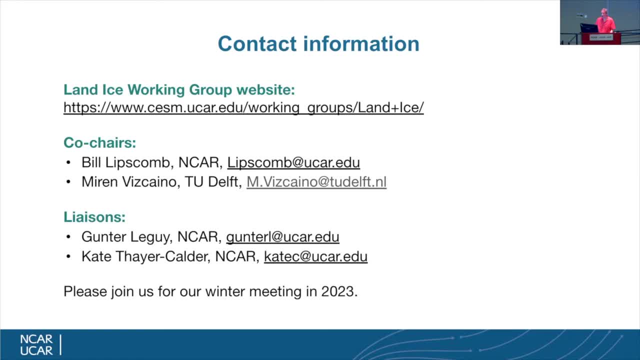 that we're looking at right now is the ice sheet model. that we're looking at right now is the ice sheet model Earth mechanism we're missing is if you have, let's say, a massive deglaciation in the northern hemisphere, which is very quick, then you can raise sea level around Antarctica a lot. 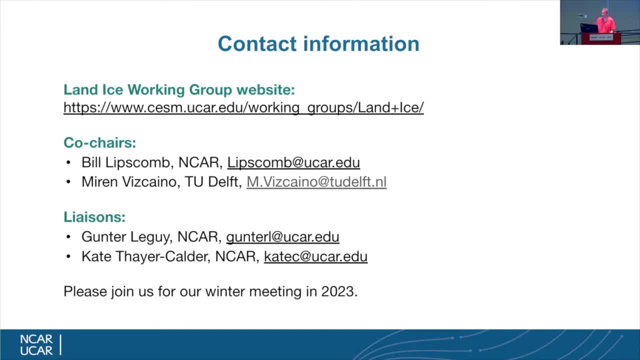 And if you do this on a time scale that's shorter than glacial rebound, then that makes it even harder for Antarctica to adjust. So you have the possibility of Antarctic collapse being triggered by what's going on in the northern hemisphere and the rate at which that's happening. 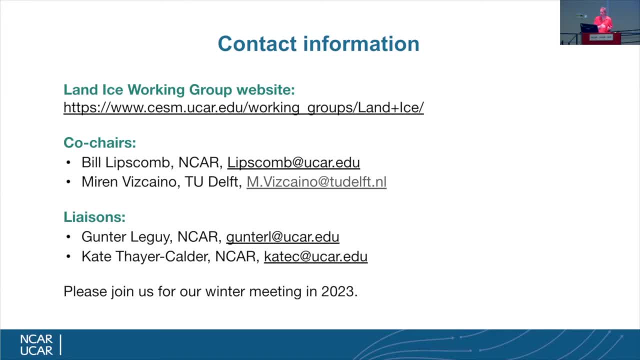 So you have a combination of external sea level rise from the northern hemisphere and potentially local ocean warming and atmospheric warming and changes in winds all going on at the same time And very challenging to untangle all those, but very interesting to work on, So maybe we should talk afterward. Yeah, I'd like that.